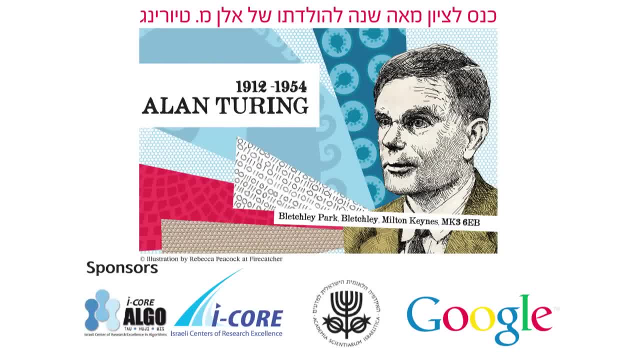 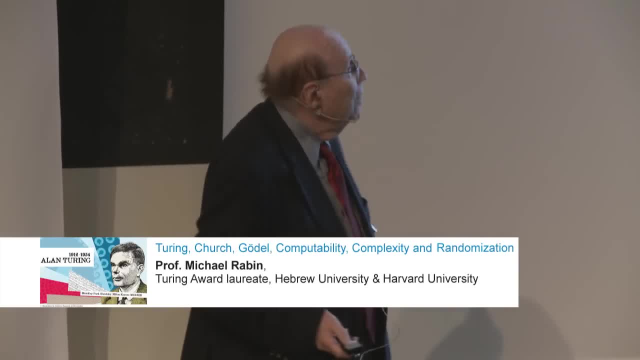 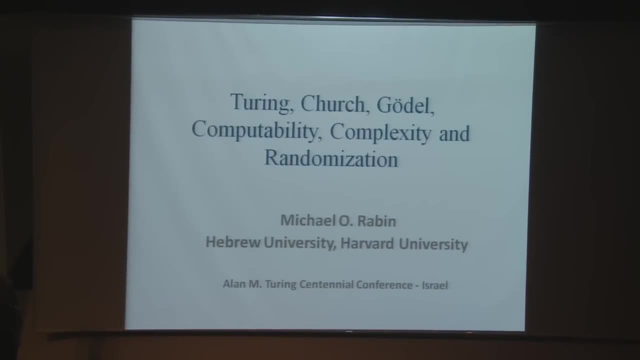 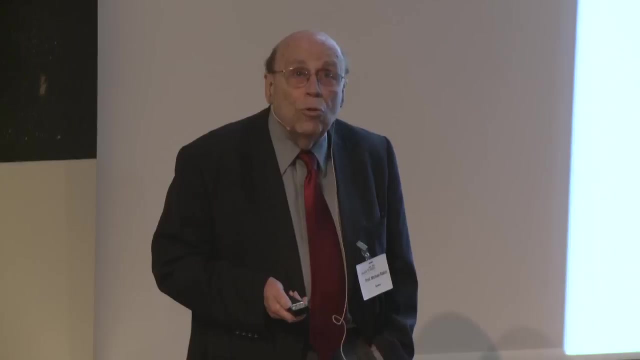 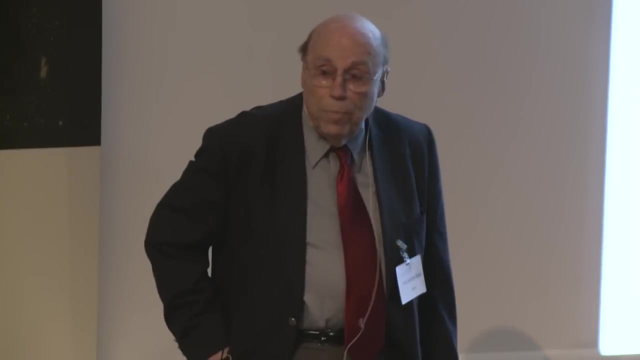 It's a great honor to have been invited to this big affair memorizing Alan Turing. I'm going to talk about Turing Church, Gödel, the topics which appear here, And the idea is going to be to give the intellectual history of the technology which is so prominent nowadays. 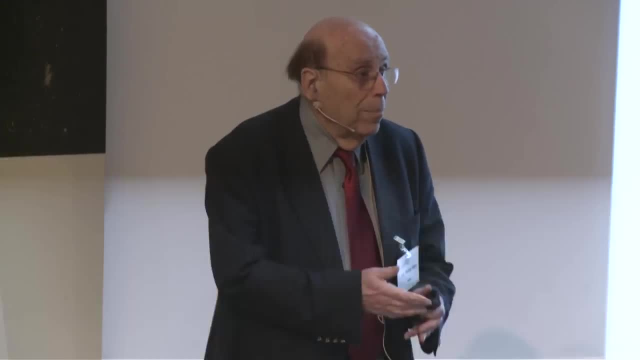 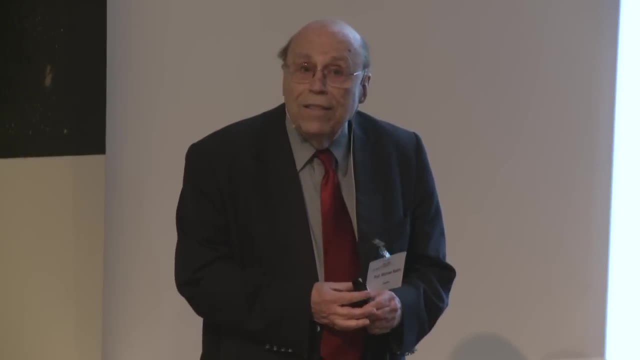 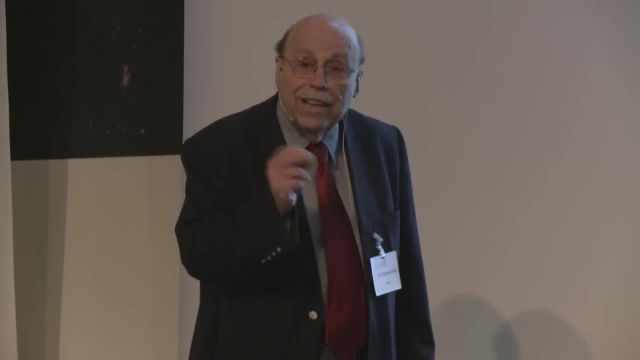 in all of our lives. all over the world, Billions of people are now involved and are using computers in one way or another, And it all essentially originated with a mathematical idea. It's an example, a prime example, of a mathematical idea. 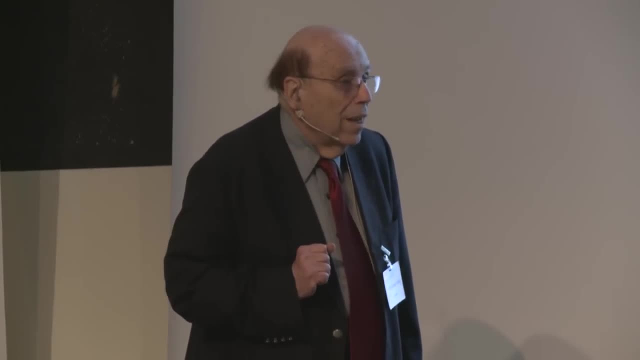 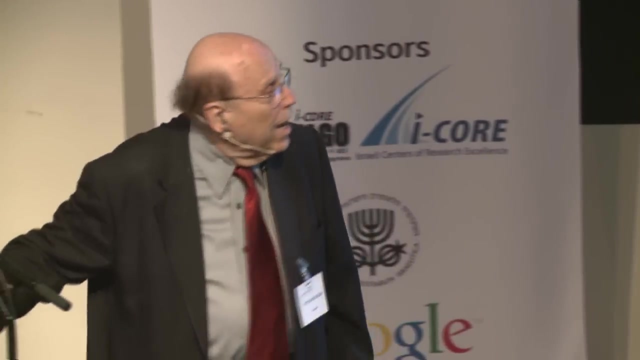 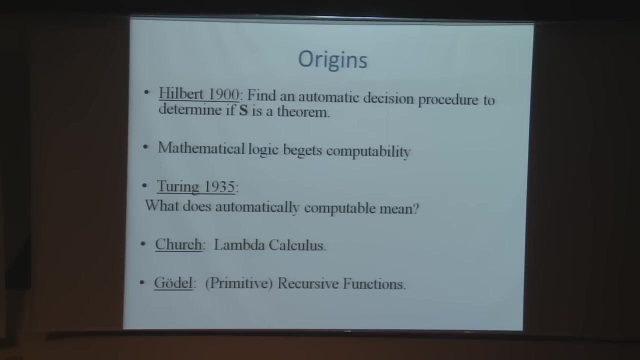 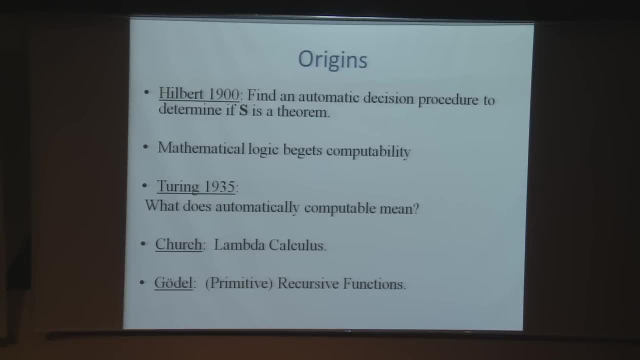 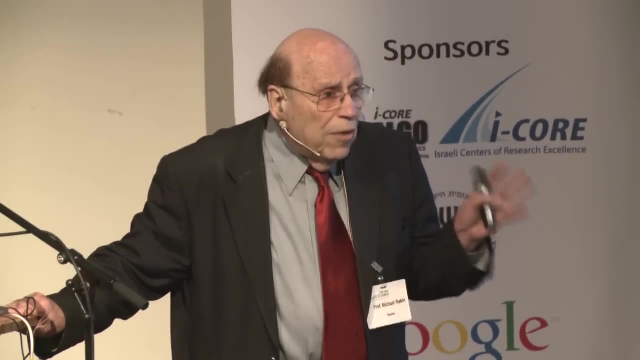 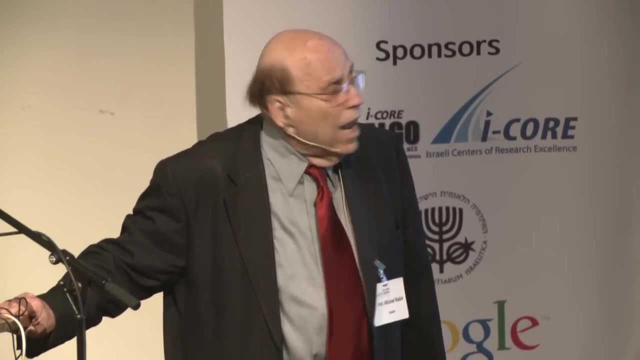 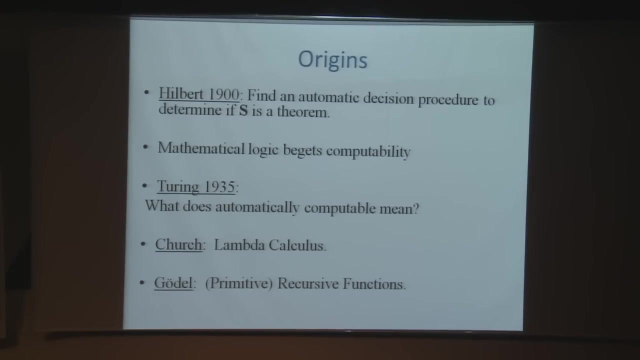 of the revolution After the year 1900, around 1900,, Hilbert posed the following question: After the formalization of mathematics by means of logic and axioms and the like, he asked, can one find an automatic decision procedure, an algorithm in today's language? 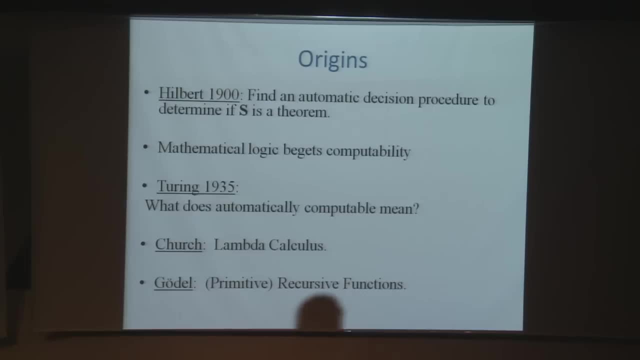 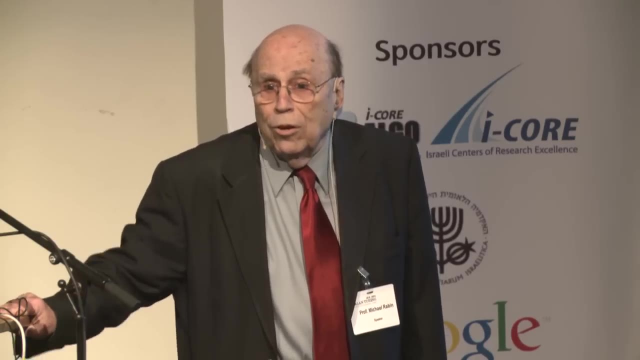 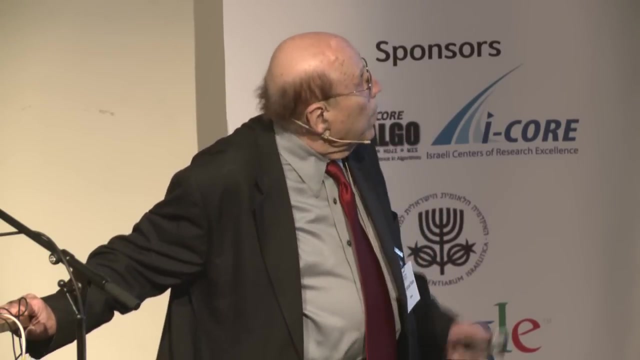 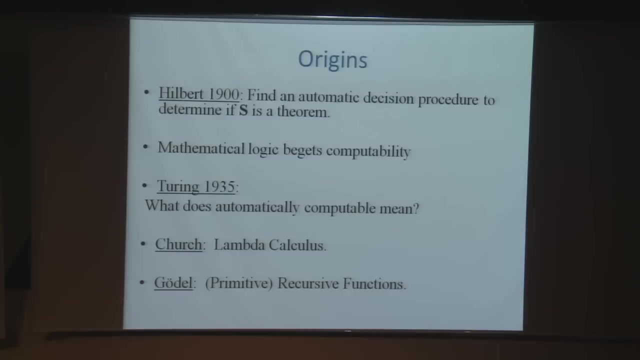 to determine, for every formalized sentence S, whether it is a theorem in a certain mathematical, let's say in set theory, or in number theory, in some algebra, in some mathematical domain. So it's really the situation that mathematical logic is the mother of computability. 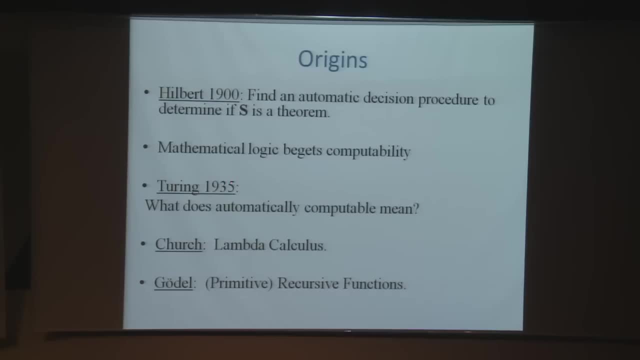 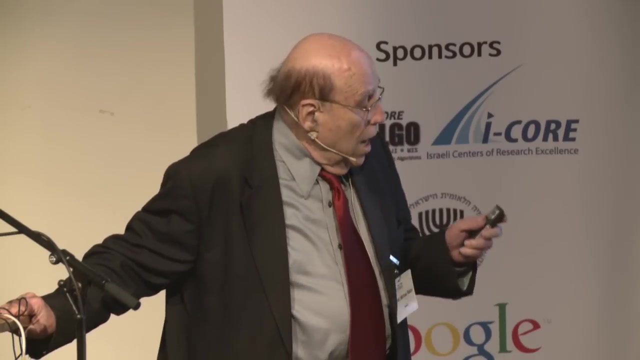 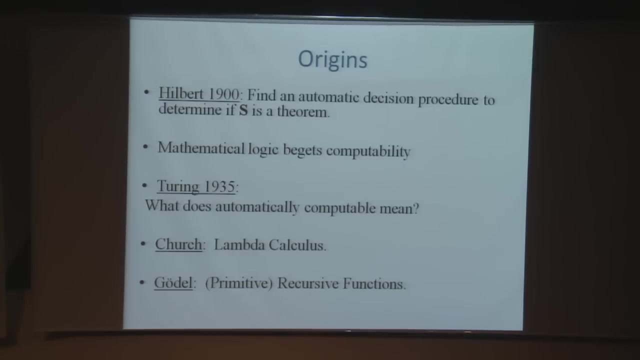 Now Turing in 1935, asked what is really meant by being automatically computable. This was left vague in Hilbert's question, And then there were three answers to that question. Turing came up with Turing machines, which I'll discuss in a moment. 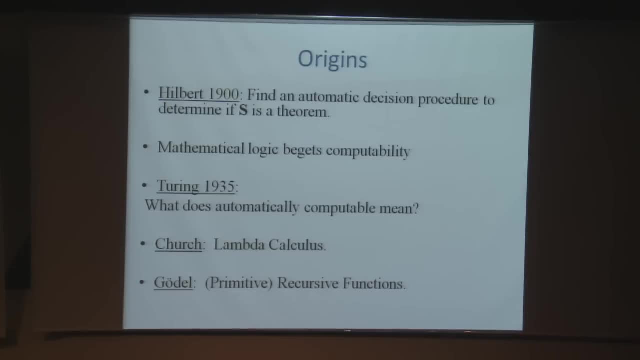 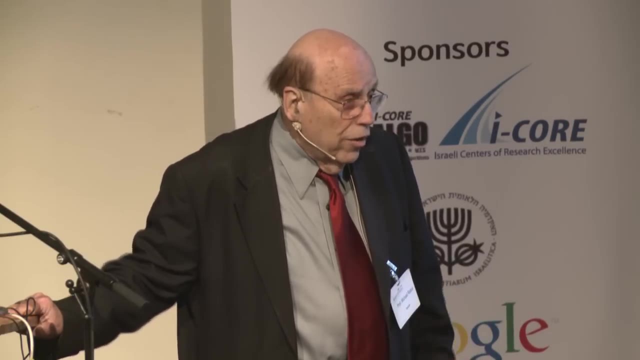 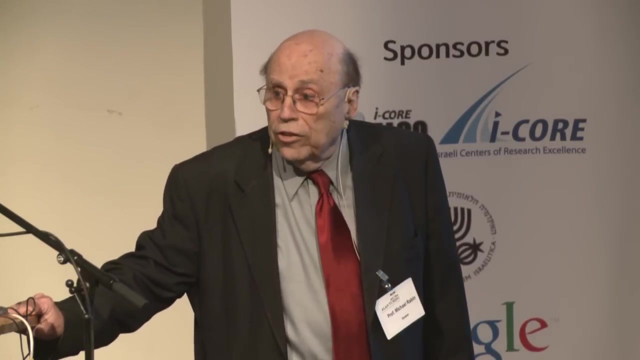 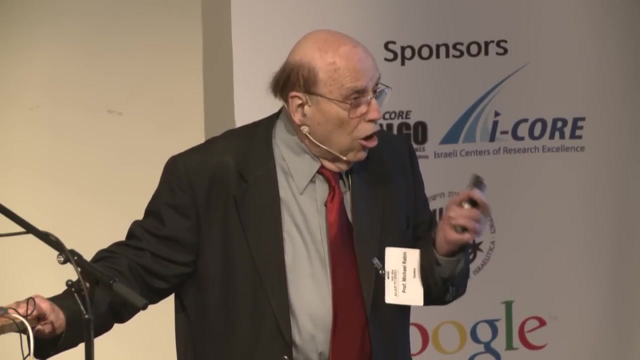 and a church independently invented the Lambda, calculus and Gödel in a different context, defined first of all primitive and then essentially general recursive functions, And it was very important that those three definitions actually in content led to the same concept. 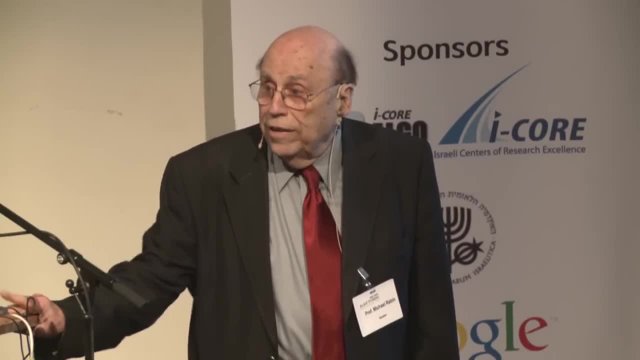 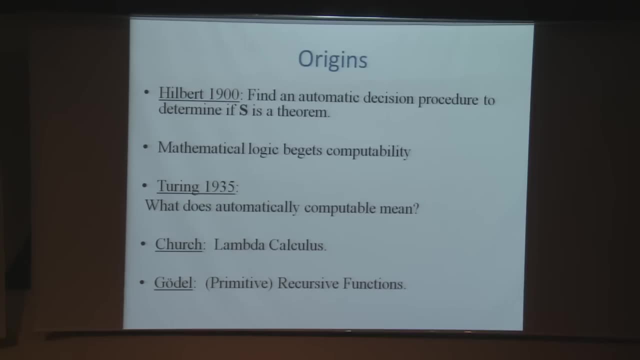 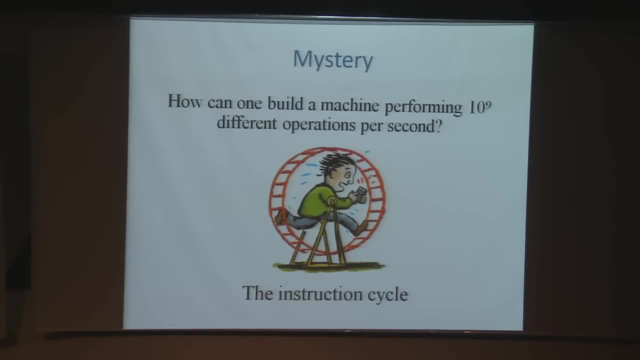 to the same class of functions, And this is is, to this day, considered a demonstration that these answers really are the appropriate answers to the question. Now we have these computers and they perform, let us say, a billion in Hebrew, a milliard. 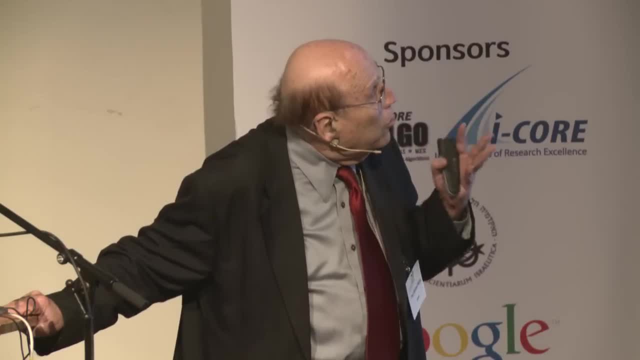 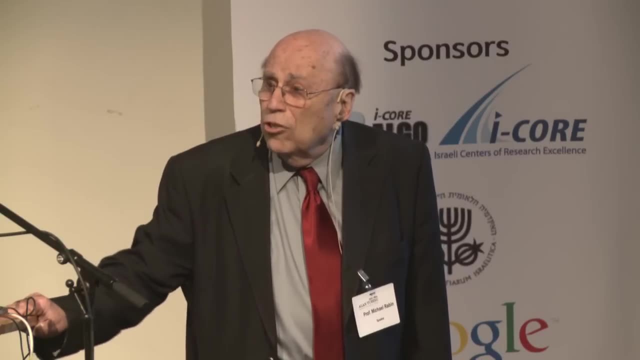 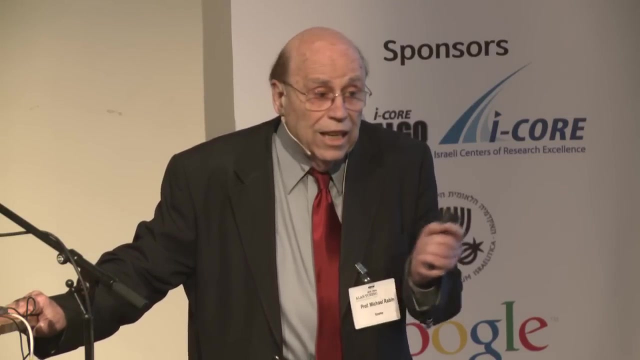 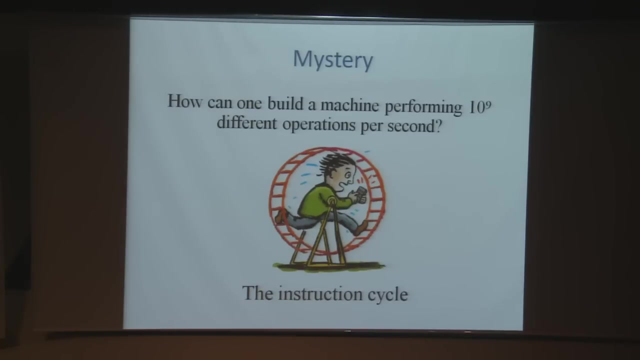 operations per second. How is it possible to build a machine performing 10 to the ninth different operations per second? The idea, the solution lies in an idea which also goes back to Turing, of actually having an instruction cycle. So if you consider a wheel, in principle 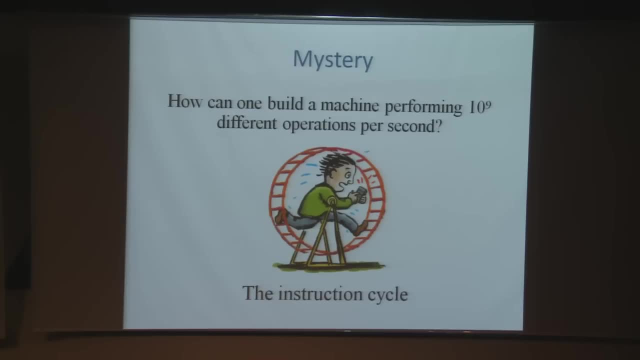 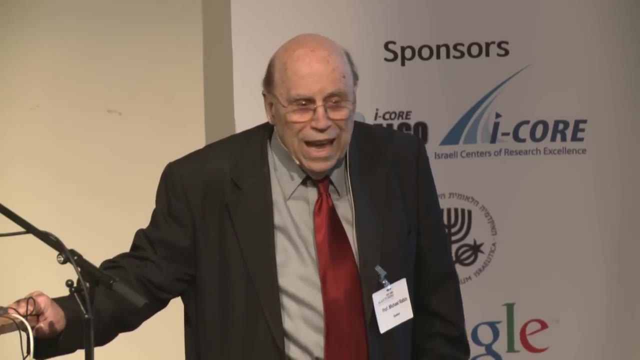 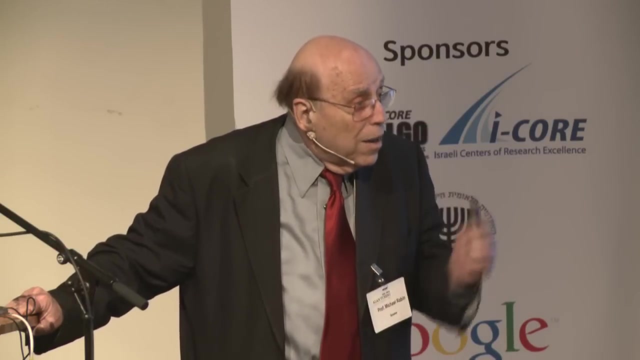 is possible to be turned 10 to the ninth times per second, except that centrifugal. centrifugal forces would tear it apart. But our computers do, paradoxically, the following 10 to the ninth times. they are doing the same thing, they are repeating an instruction cycle. 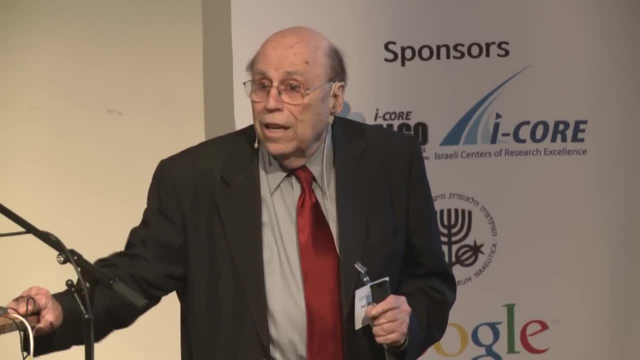 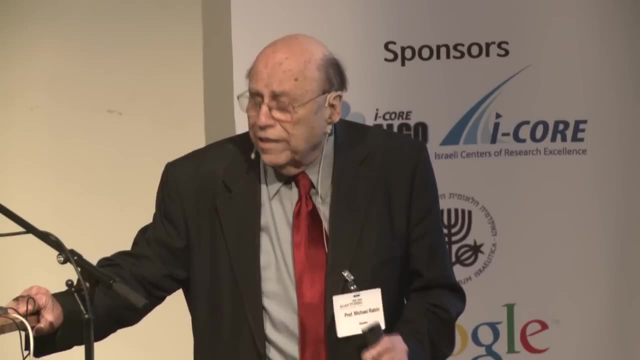 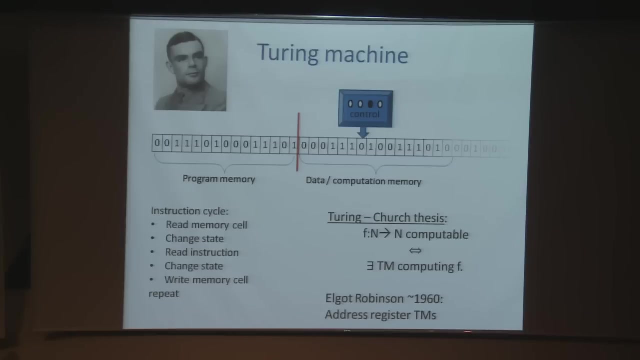 But each time an instruction cycle is being repeated, a possibly different instructions, actual instruction is being performed. Now, Turing machines. The most readily understandable definition of computability is via the construct which we now call a Turing machine, And the Turing machine has the following components: 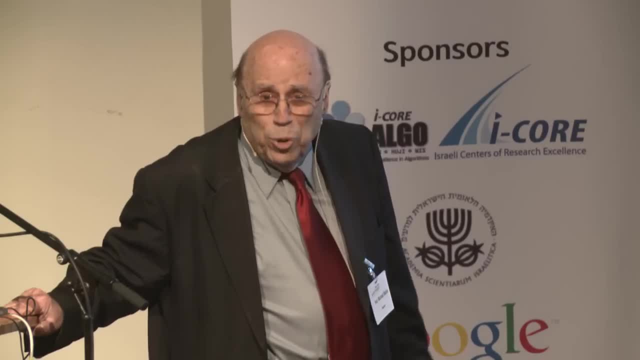 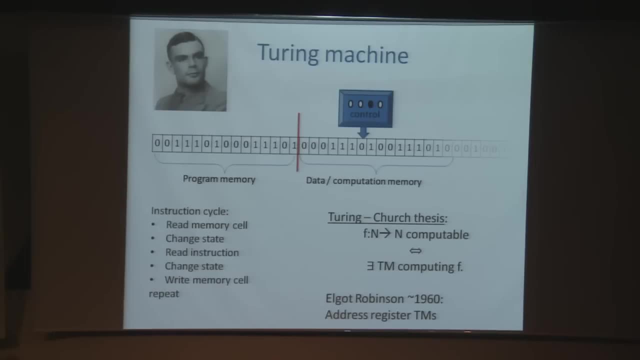 The memory is a tape which is a potentially infinite secret sequence of memory cells, And that tape- and this goes back to Turing- is divided into a section where the program is being stored. This is what you have on the left there, the program memory. 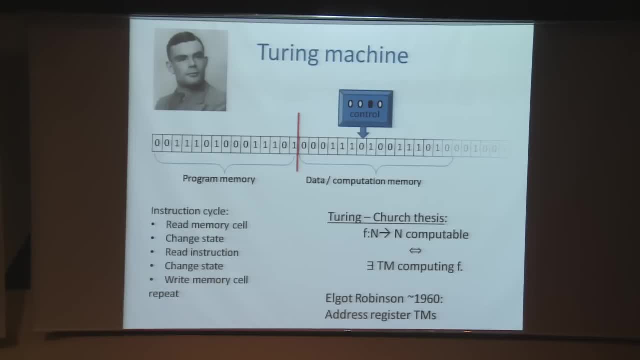 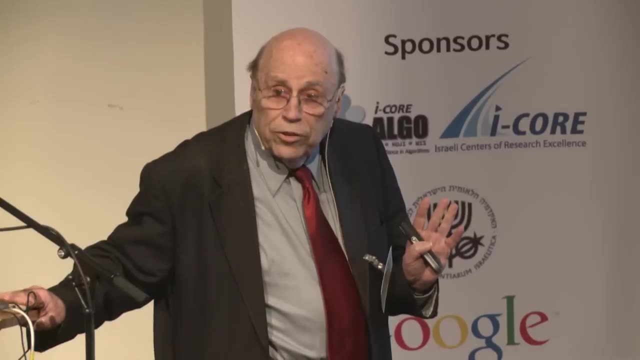 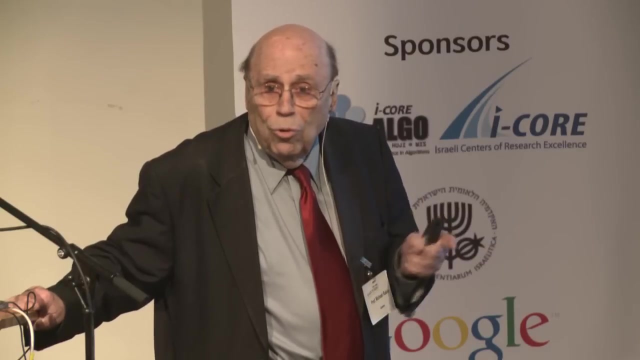 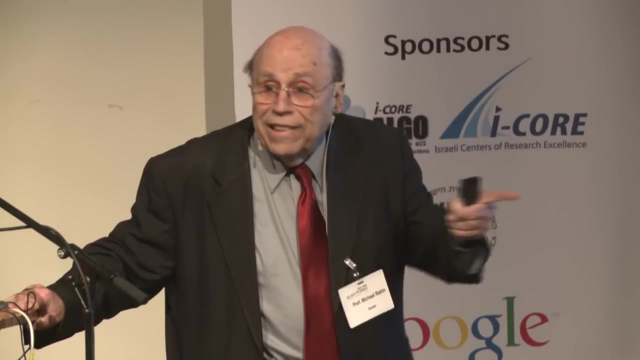 And then a part which is the data and computation memory. Now, if you look at modern computers essentially, if you look at modern computers essentially, the memory there, especially, you know, with virtual memory, is essentially still logically an extendable sequence. 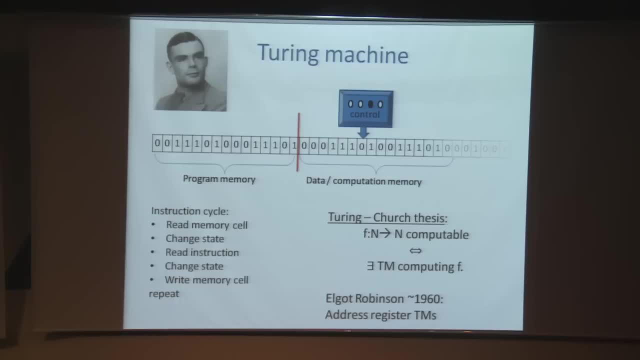 of memory cells which are being addressed by the address register. Now, the way he conducted the computation is to have the instruction cycle, Namely, it starts by reading a memory cell. So here we read a memory cell, Then you change state. 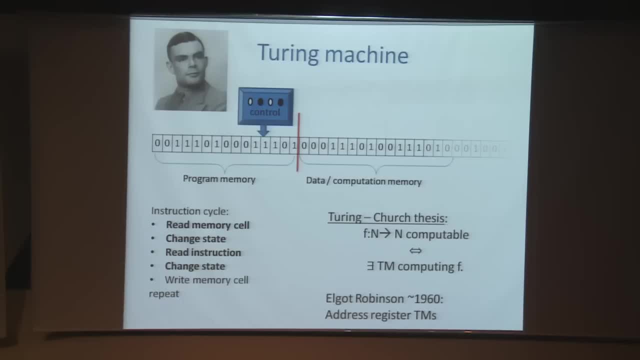 You read an instruction. you go to the program, you read an instruction, you change state, You go back, you write the memory cell And then you repeat, And then you repeat, And then you repeat. That's the instruction cycle. 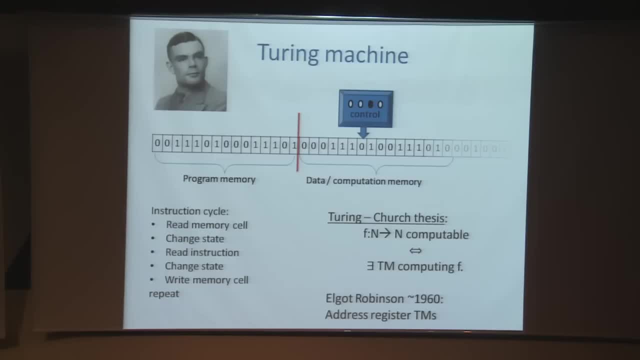 So the Turing Church thesis was that being computable is equivalent to having a Turing machine computing that function Now Turing. for his construction had the tape and had the control move, which was a sort of one step at the time. 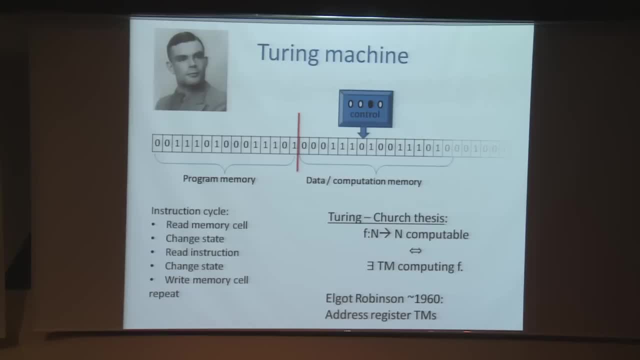 In 1960, look at the bottom of that slide here. In 1960, look at the bottom of that slide here: Elgort and Robinson at IBM, Carl Elgort and Abraham Robinson had a version of the Turing machine. 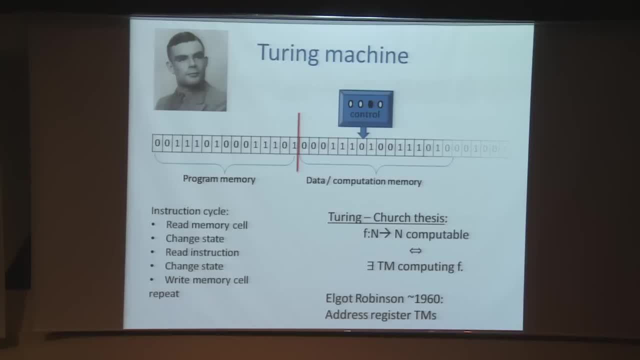 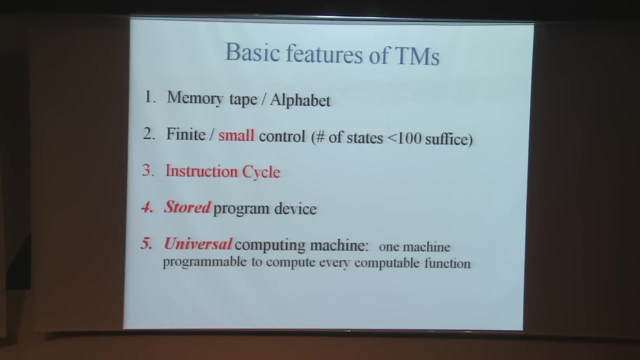 which has address registers. So very much now, very close to what we have nowadays. So moving on. So moving now to the next one. what are the basic features of a Turing machine? There is a memory tape, That's this extensible sequence of memory cells. 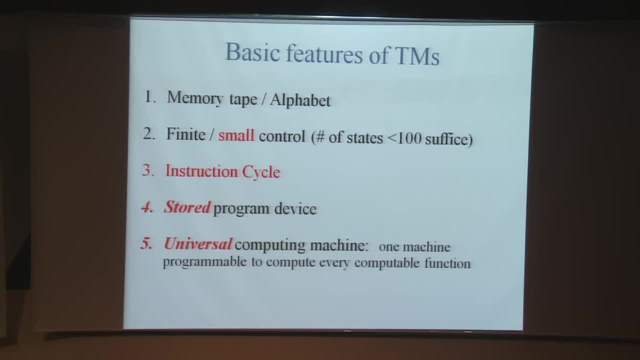 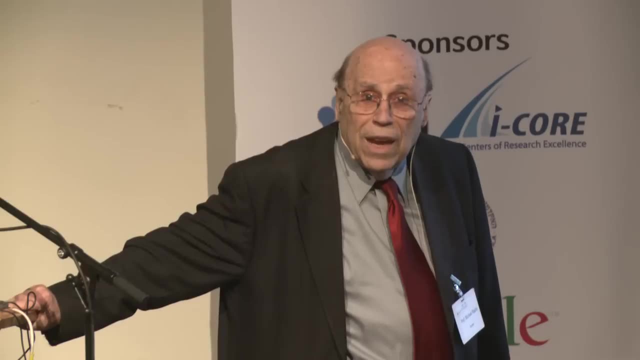 Then, and this is the point which is very often overlooked- there is a small finite control processor. There is a small finite control processor. You see, we could sit together and see the memory tape. You see, we could sit together and see the memory tape. 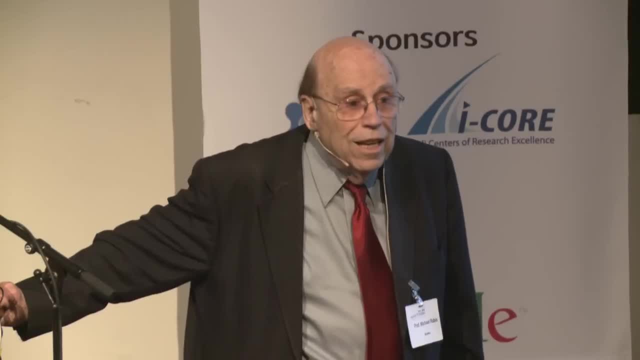 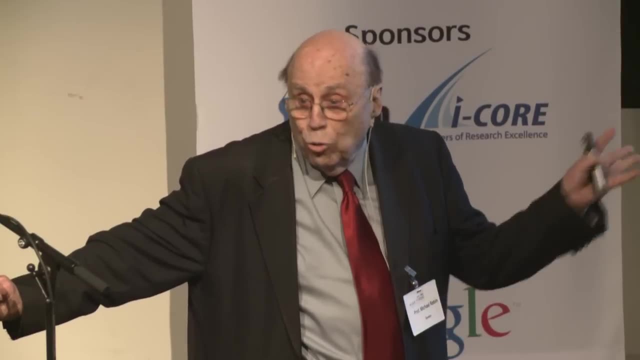 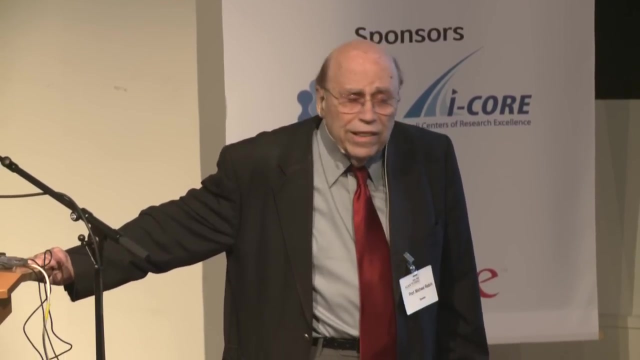 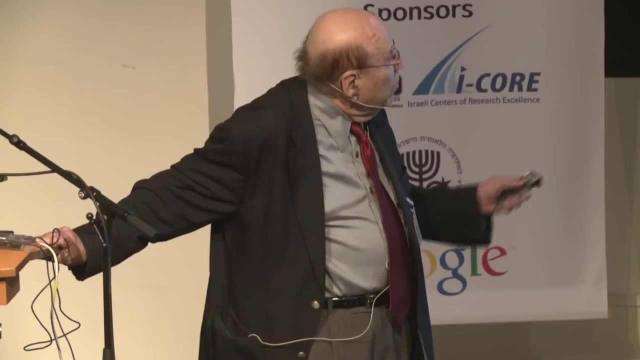 together, I and any three of us here, and devise a universal Turing machine, a universal computer using no more as Turing did, no more than maybe 50 or 60 different instructions. What's the significance of this fact, If it would turn out that to have a universal machine- and that's here the fifth point- 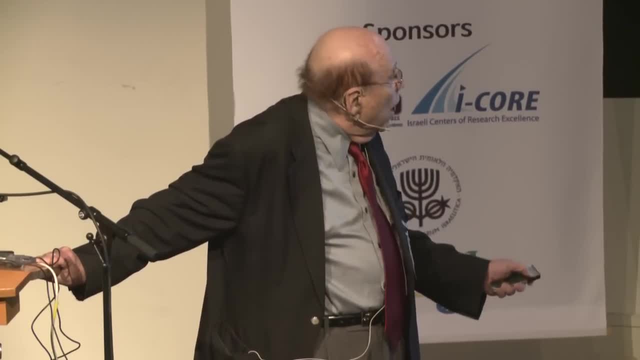 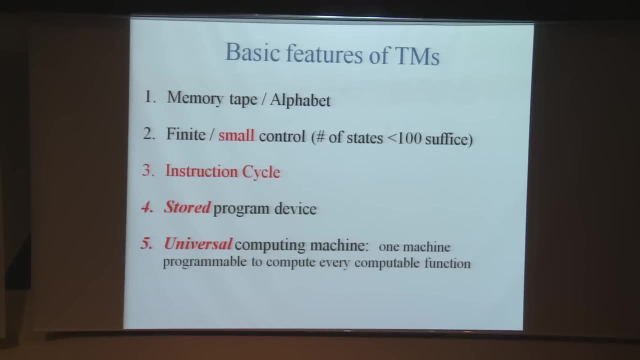 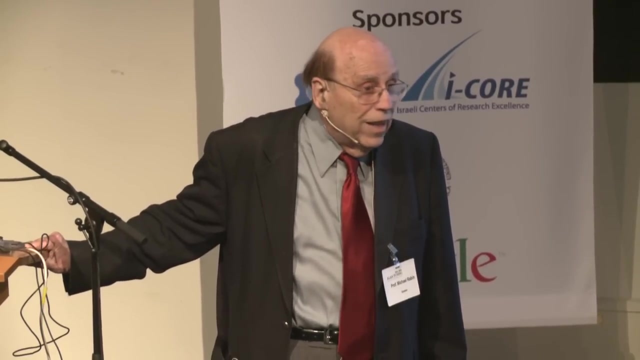 to have one machine which can be programmed to calculate any computable function. if that would have required, let us say, 20,000 instructions, then in the early, in the late 40s and early 50s, with the technology then available, maybe even with the technology now available it. 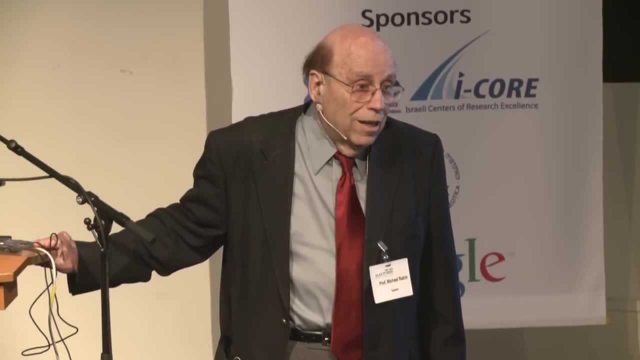 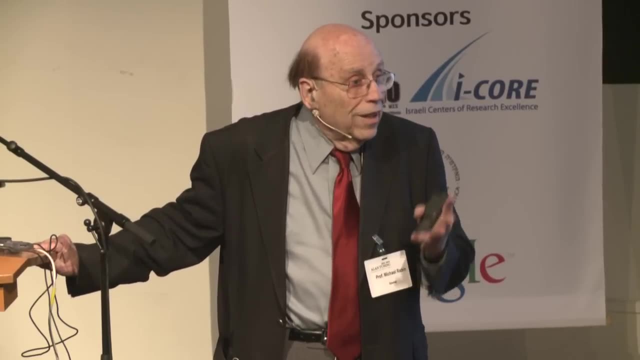 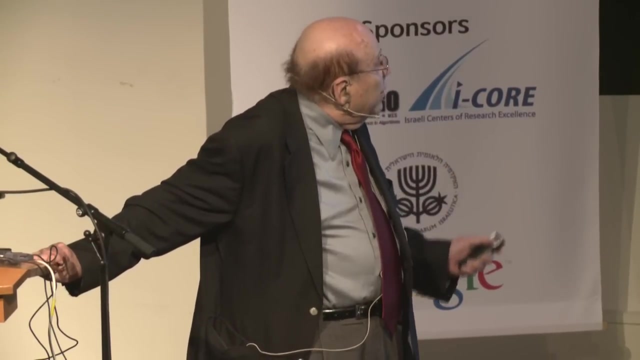 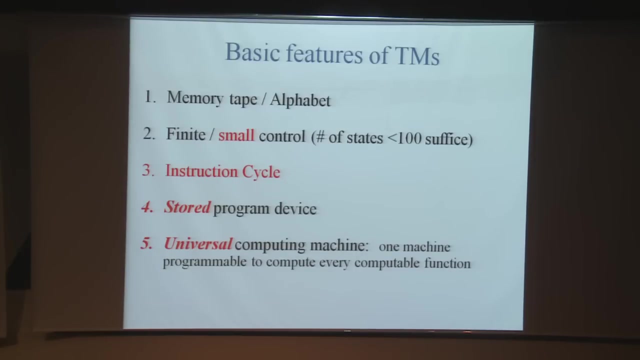 would have been impossible to build a universal computer. Okay, So this is an extremely important point, sort of uncovered by Turing in his original work. Then the next thing is that the device is a stored program device. The program, the control- and I'll get back to that point in a moment- is in the same. 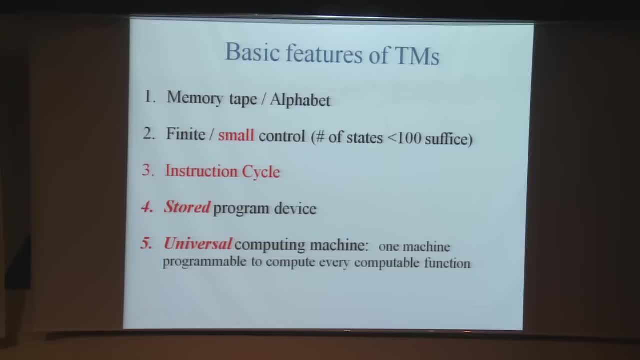 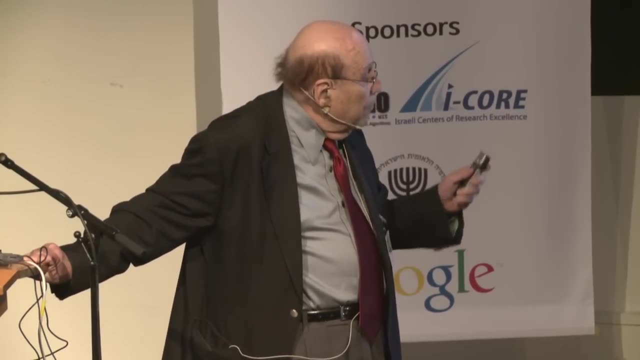 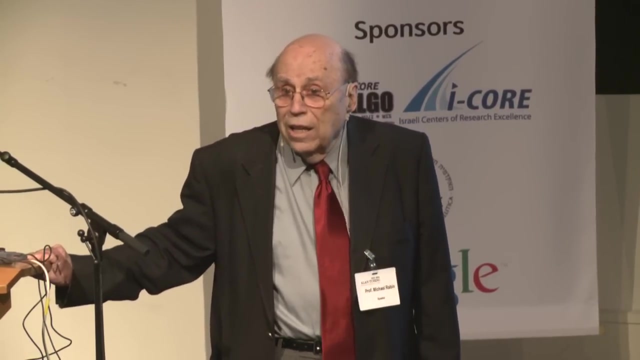 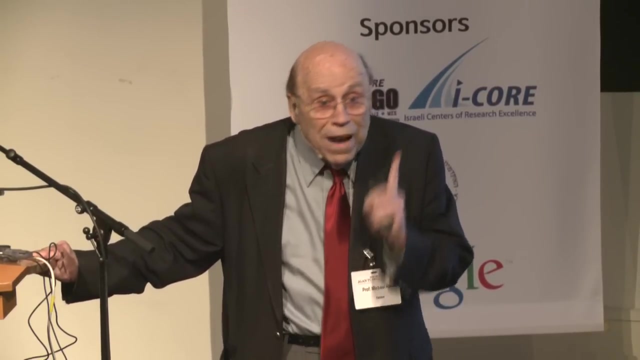 memory, where the computation in the same fast memory nowadays, Where the computation is being conducted. And finally, unlike the computing machines suggested, say, by Pascal and Leibniz, which did additions, multiplications and so on, this is a universal machine. 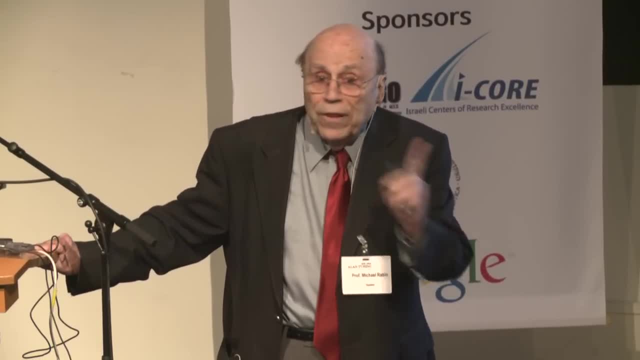 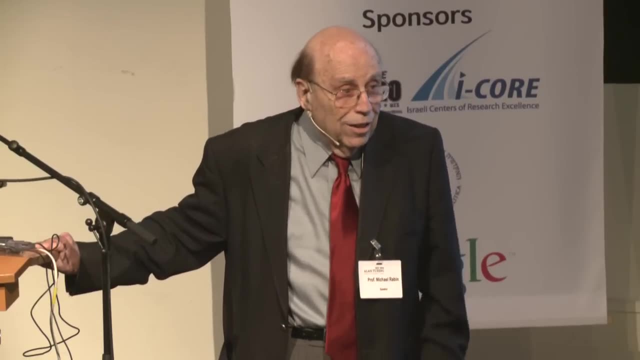 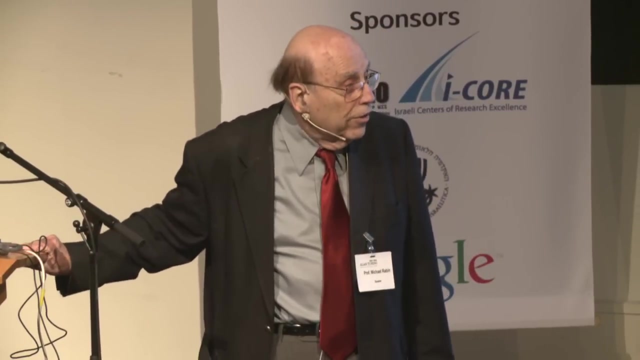 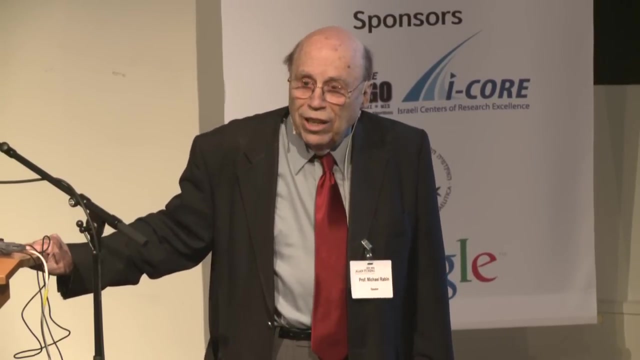 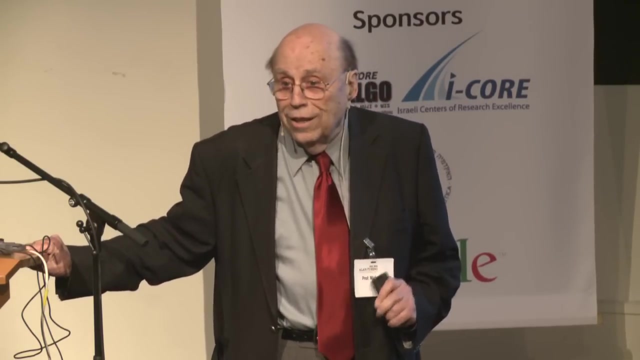 One machine which, by different programs, can calculate any computable function. One machine, One machine can do it, And these are the essential features of the processor that we have in all of our devices. So, essentially, Turing gave the intellectual blueprint for what we could call in sort of 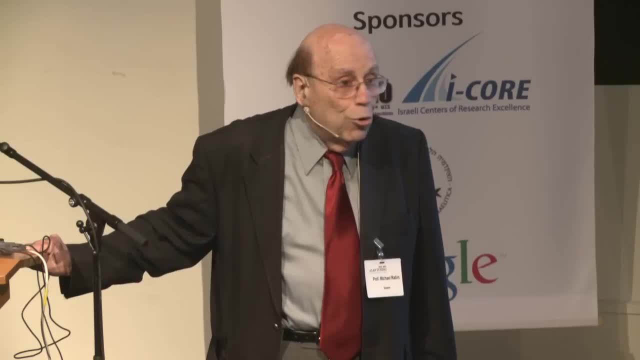 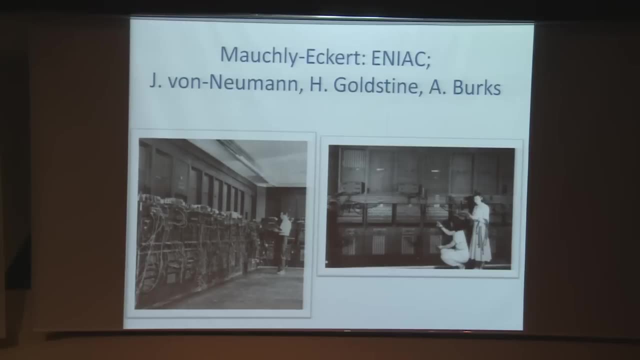 children's language, the little engine that could. Okay, All right, Now let's go back to history, to essentially the first large computer that was constructed. Moakley and Eckert constructed the ENIAC, And then I'll in a moment come to John von Neumann, Goldstein and Burks. 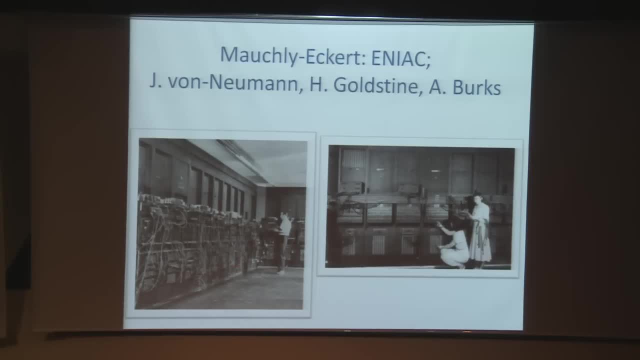 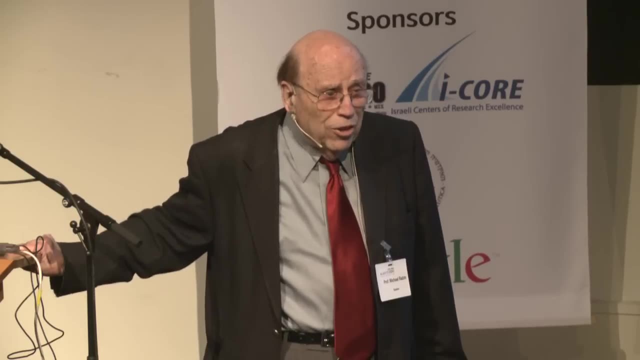 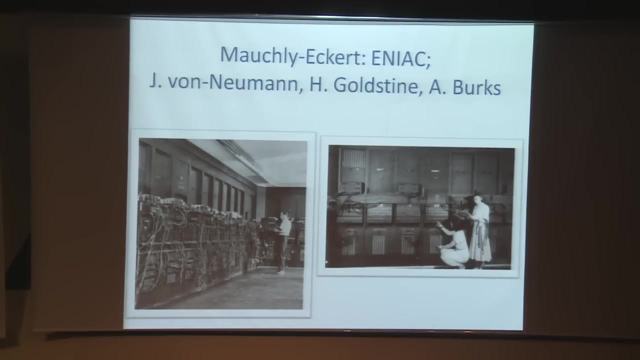 Now, this was an enormous machine. Here you have it. It was electronic. It could perform Maybe, Maybe, a thousand or so computations per second. And now, how was it programmed? It was programmed by going to the control board, plugging wires and moving and switching. 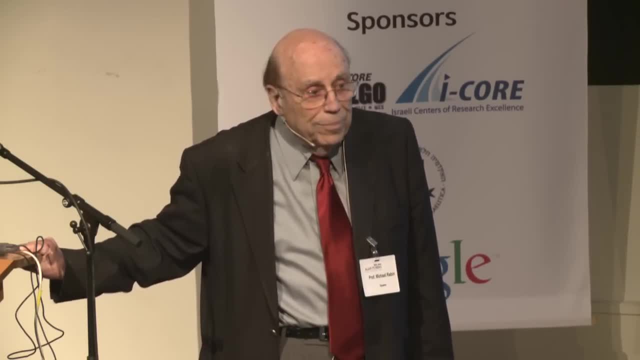 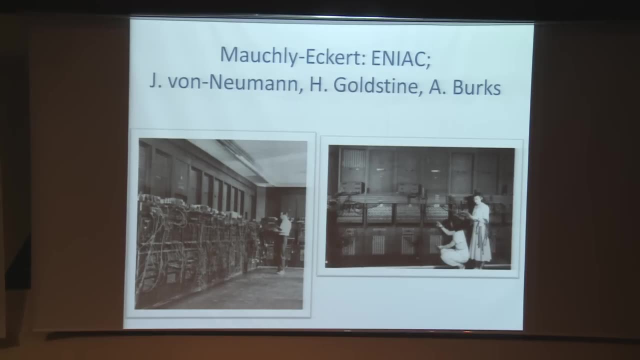 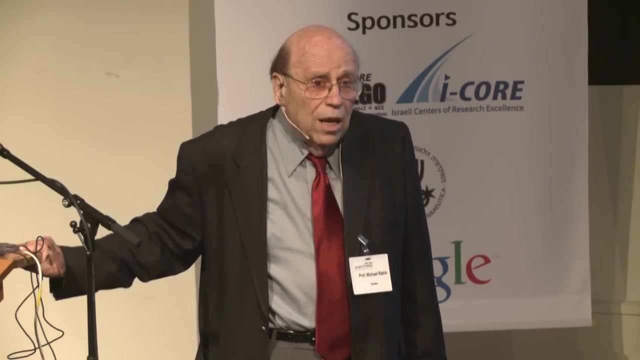 sort of switches. You see these two women standing there and they are doing the work to sort of reprogram the computer. Now how does von Neumann come into it? This machine was built for the purpose of doing computations for the army, to calculate. 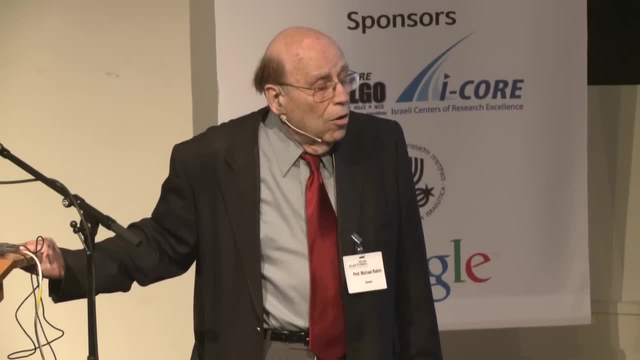 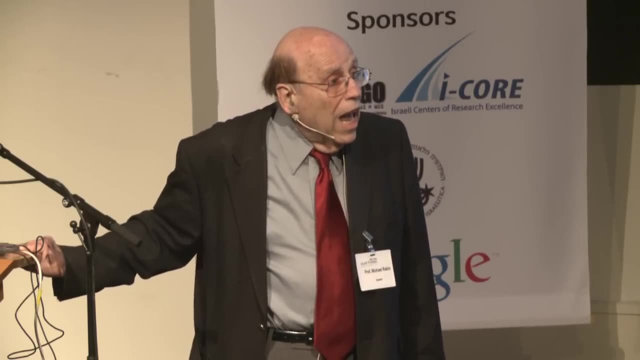 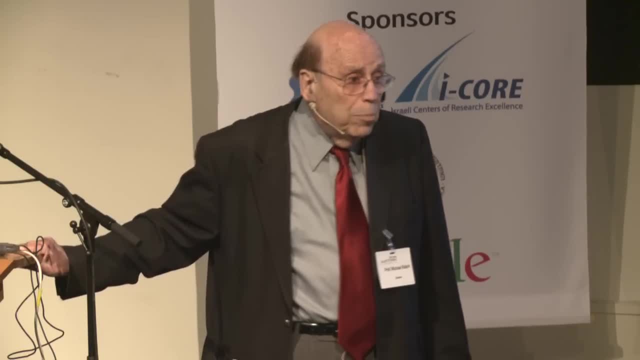 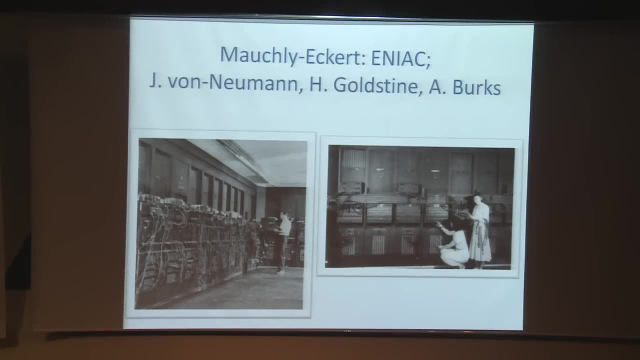 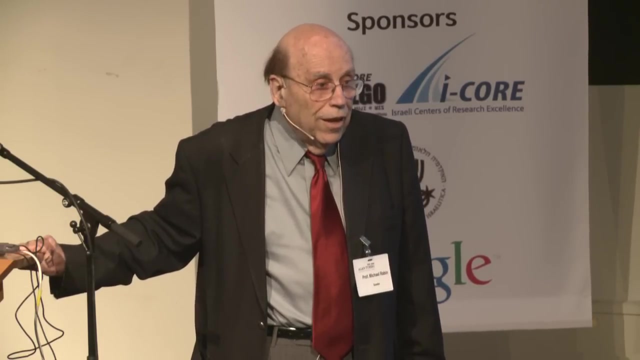 And von Neumann and Goldstein were working at the Aberdeen proving grounds doing computations for the same purpose. So, and this I have personally from Hermann Goldstein, He took von Neumann to see the ENIAC machine And von Neumann looked at that monster. 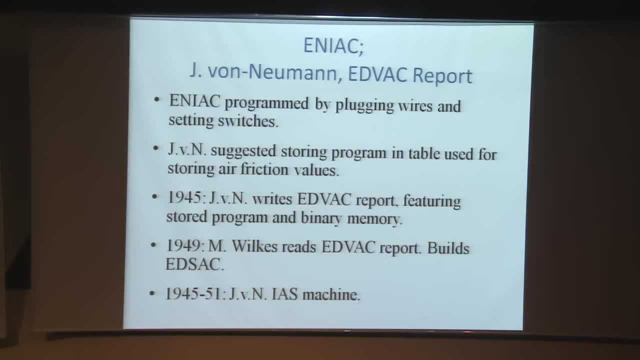 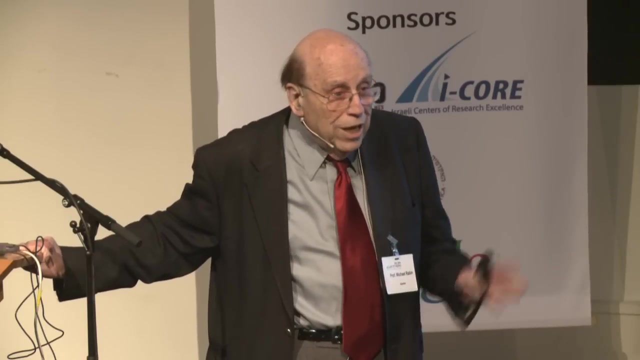 Now this machine. This machine, So the ENIAC was programmed by plugging wires and setting switches. Now von Neumann, when he was visiting there, looked at that machine and the machine had a primitive electronic memory storing a table which contained air friction values, which 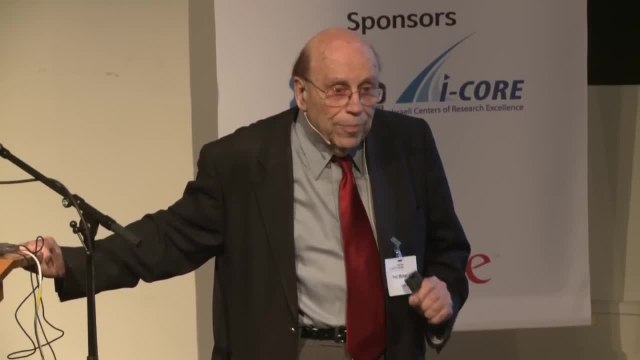 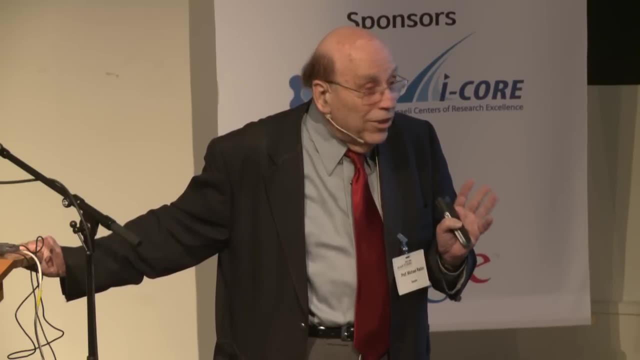 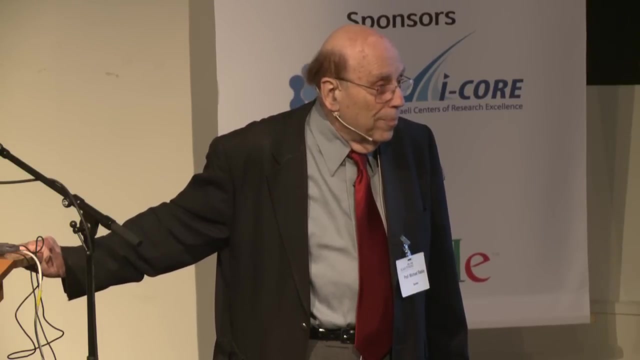 you needed in order to calculate those trajectories. And he, as he was standing there, the man was a clear genius von Neumann- As he was standing there, he said: why don't you store the program in that table and have the whole thing, you know, completely electronic? 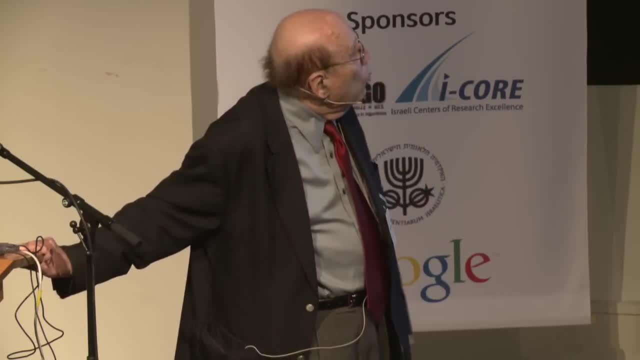 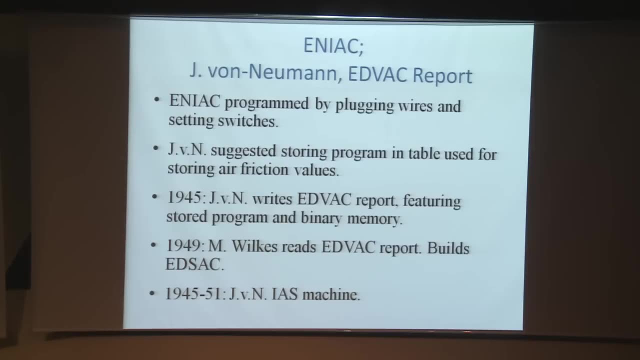 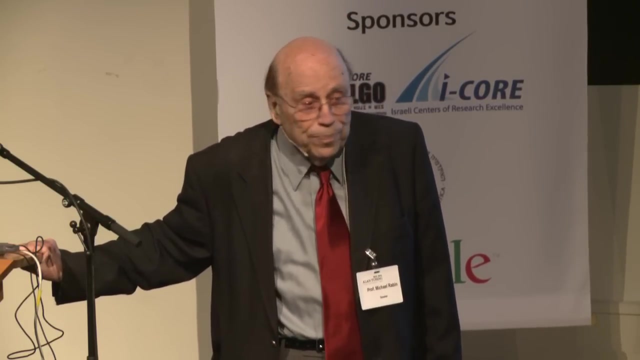 And then it can be changed by sort of reprogramming the table Now in 1945.. von Neumann, von Neumann. von Neumann wrote the EDVAC report featuring a stored program, a binary memory. Believe it or not, the ENIAC was doing calculations in decimal form. 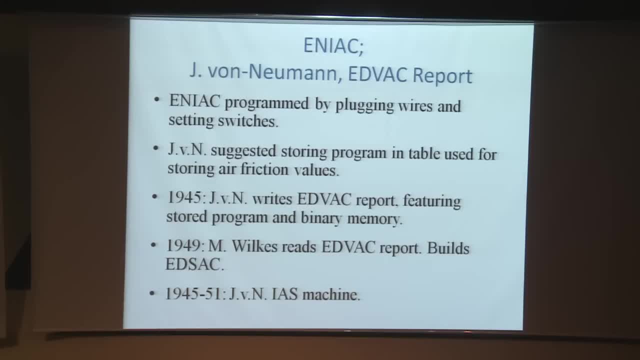 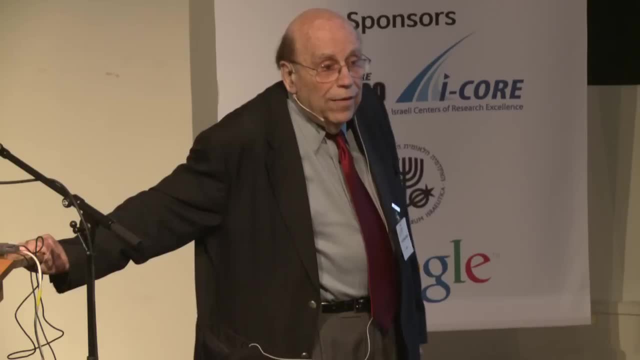 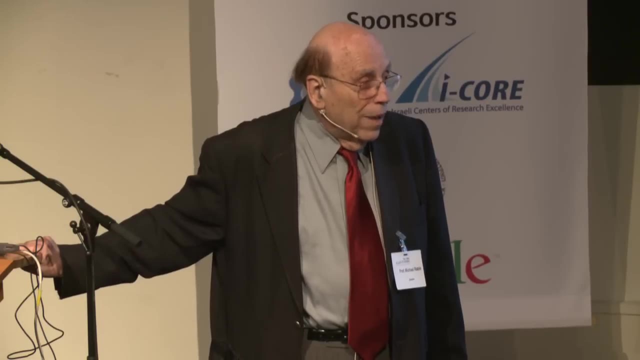 So a binary memory. And of course you know the EDVAC was scheduled to be a universal computer. Now I was in Princeton in the 50s And let me share with you my relationship. I've never met Turing, but I did meet Goldstein. 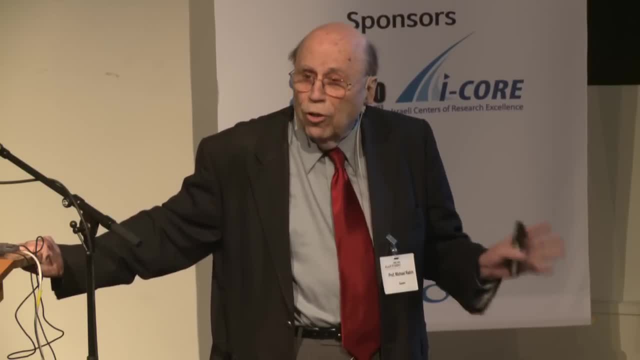 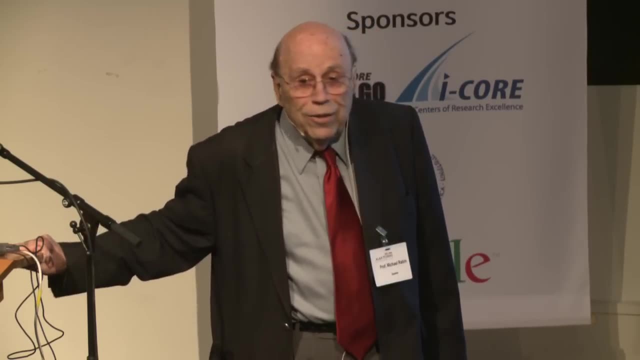 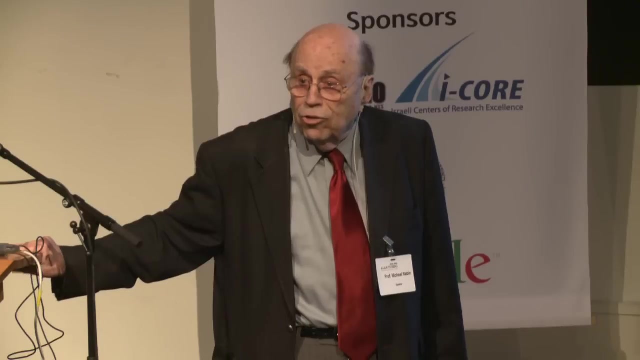 von Neumann, not von Neumann, sorry Church, of course- Gödel and a few other of the main figures. Now, in the early 50s I was a student at the Hebrew University of Jerusalem and I was working mainly in algebra and in logic. 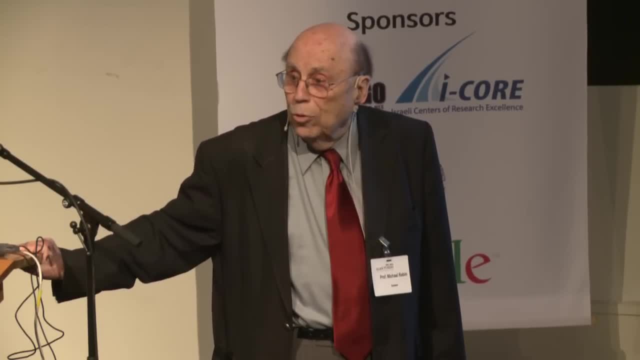 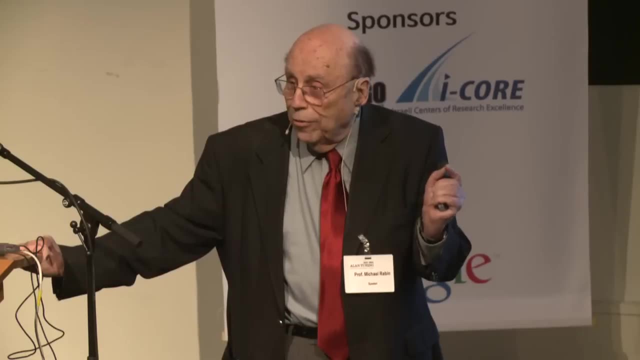 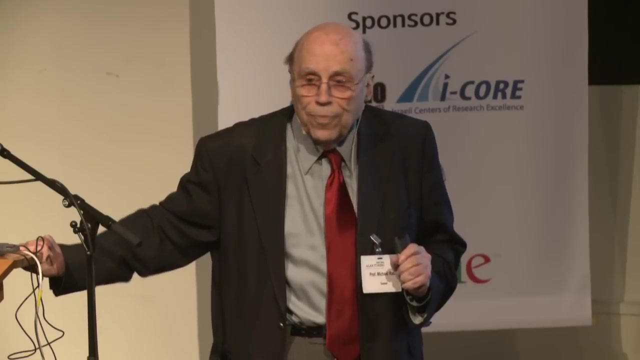 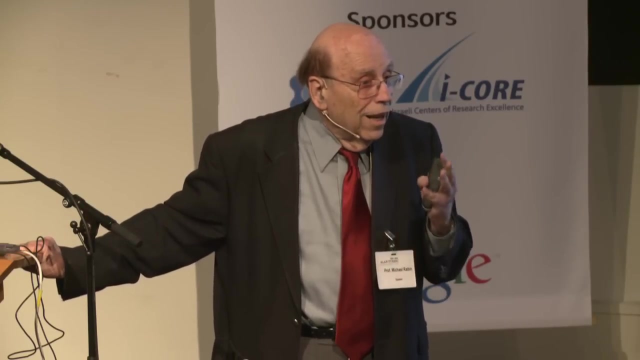 And I ran across Turing's paper. Turing's paper, It was a paper about computable numbers, And this was as computing technology was emerging. The first machines were being built by IBM, using in part also punched cards and so on, And I realized, looking at that paper, that here you have a technology that needs a science. 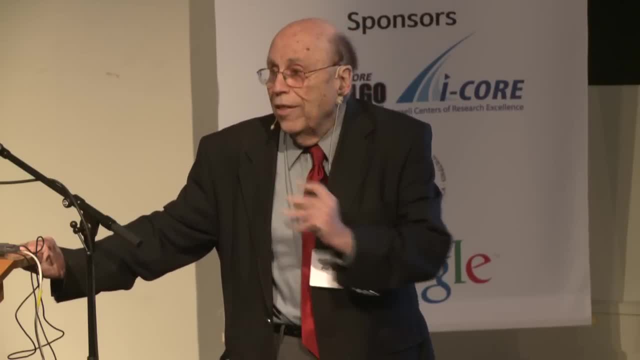 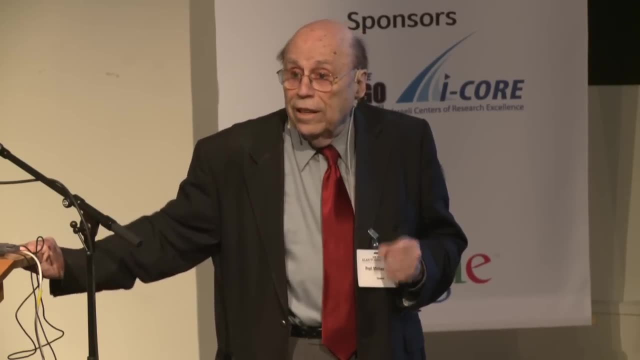 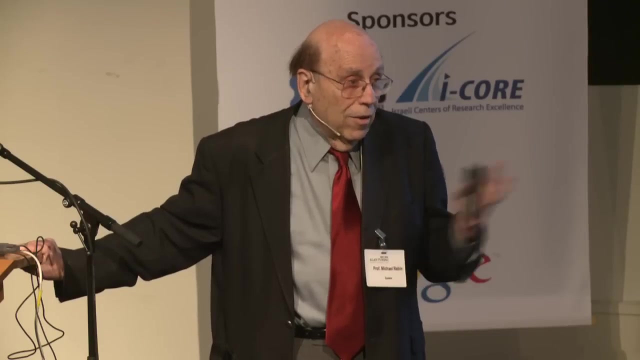 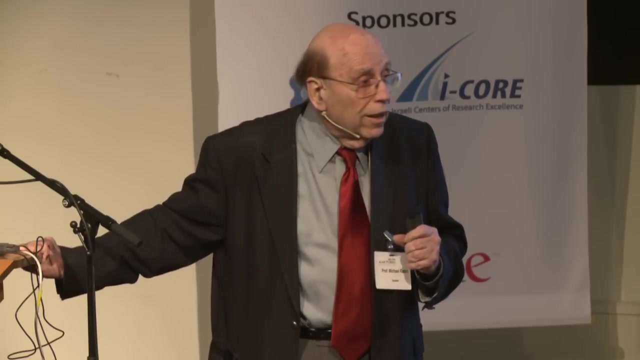 to support it. That prompts the creation of a science for science, and the center at the time was Princeton. That's where Gödel Church and the people around von Neumann were sitting at the Institute for Advanced Study. Now I have a distant relative who is a biologist. 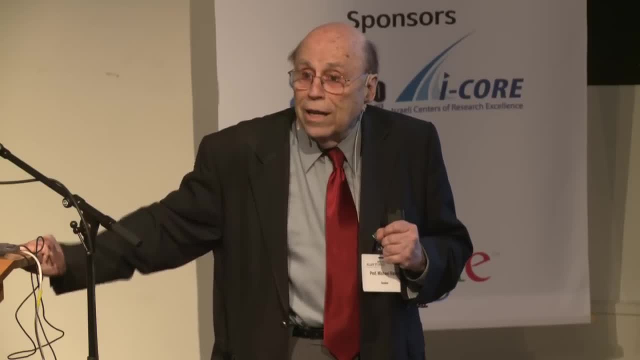 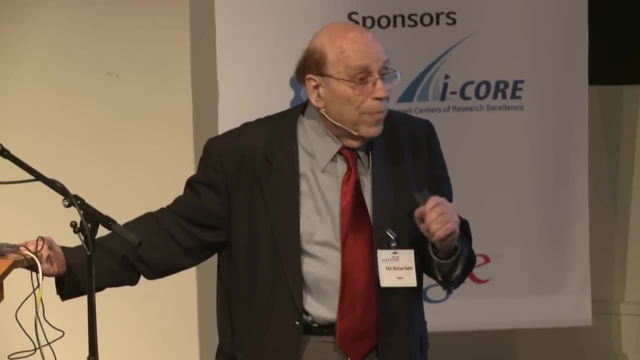 and he met me at some wedding and he said, Michael, I was 21 years old. he said, Michael, I understand you're going to Princeton. What are you going to do there? And I said: I want to study to follow. 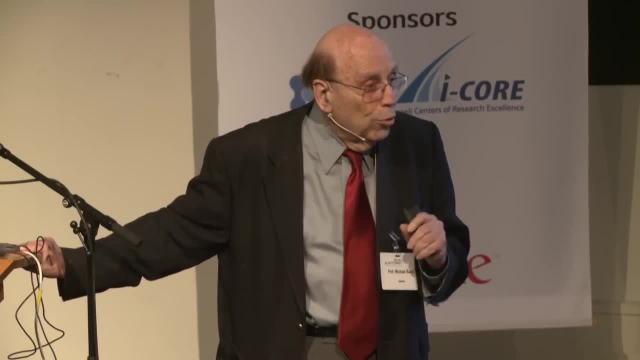 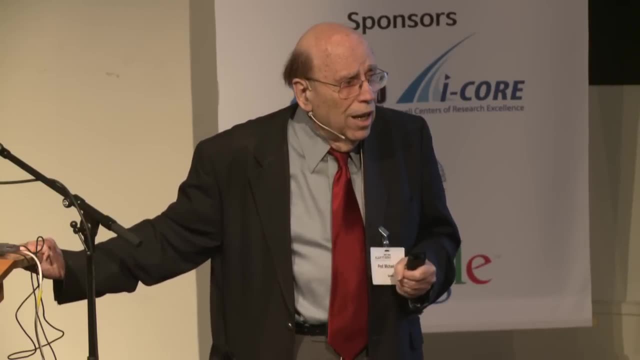 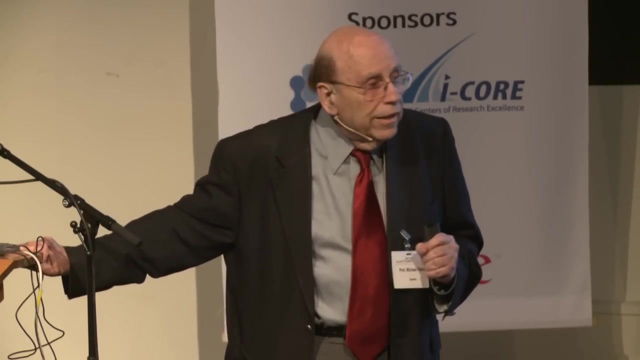 the scientific foundations of computing and computers. And he said: computers- what are computers good for, except for doing payrolls and inventories and some large-scale computations? And I said to him: you know, you are a biologist, and that was before, by the way, the double helix. 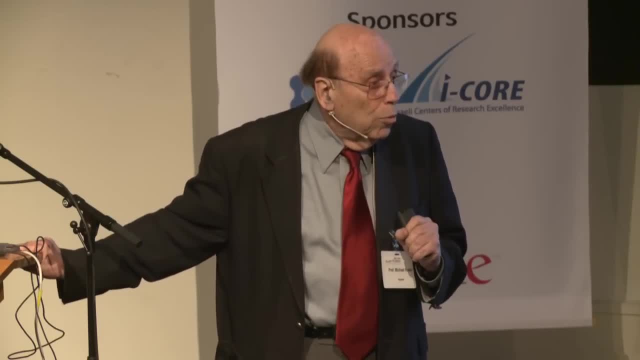 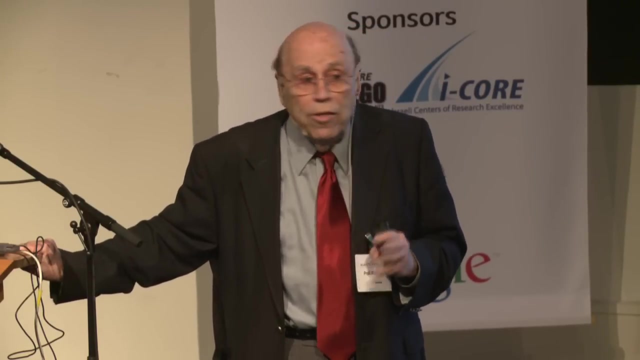 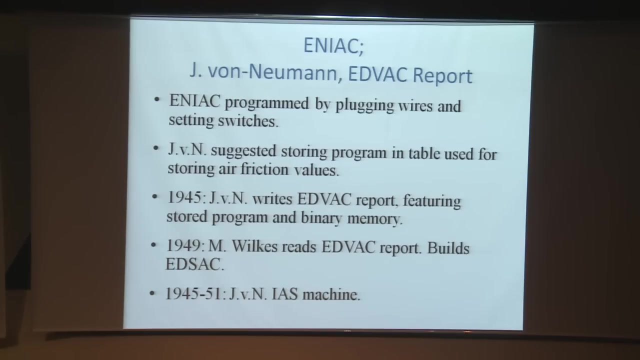 So I said to him one day: computers are going to be used to analyze and calculate the properties of very large molecules like proteins. And he looked at me almost contemptuously and he said this will never happen. Okay, so he wasn't quite right. 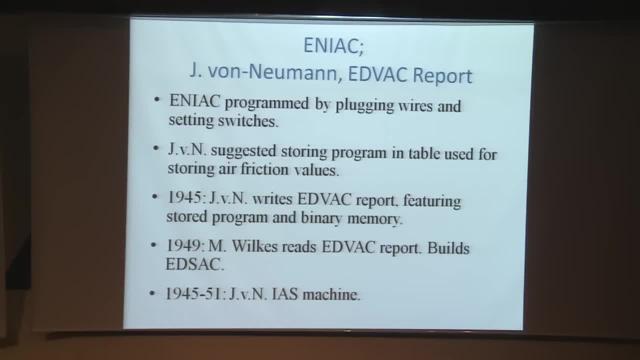 Now at Princeton. so you had the sequence of events. von Neumann writes the EDVAC report containing all the features in 1949, Wilkes in England reads EDVAC reports and builds ETSAC and from 1945 to 51,. 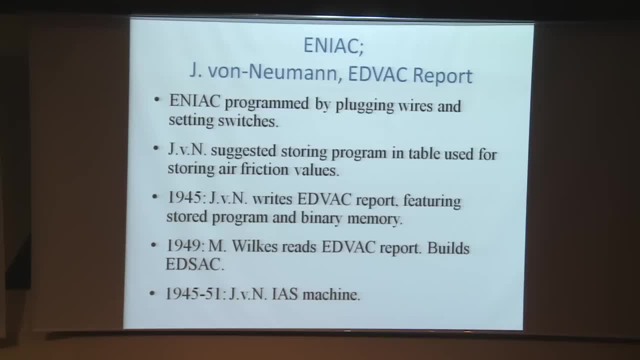 von Neumann and people around him build the Institute for Advanced Study of Computers. Now at Princeton you had the sequence of events. von Neumann writes the EDVAC report containing all the features in 1949,. Wilkes in England reads: 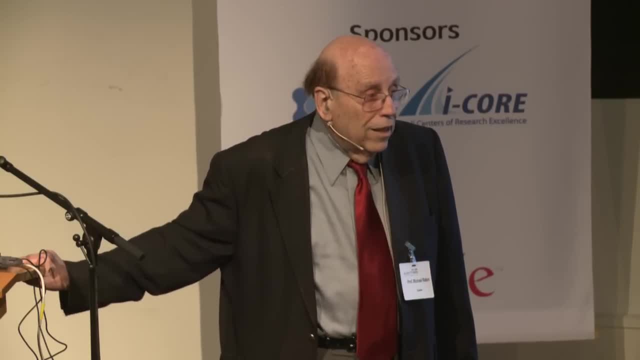 EDVAC reports and builds ETSAC. and from 1945 to 51, Wilkes in England reads the EDVAC report containing all the features in 49, Wilkes in England reads EDVAC reports and builds ETSAC. 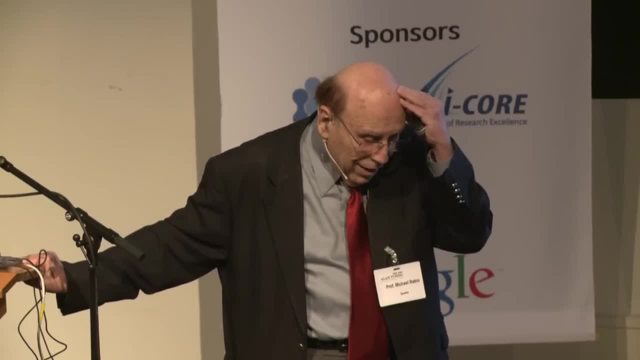 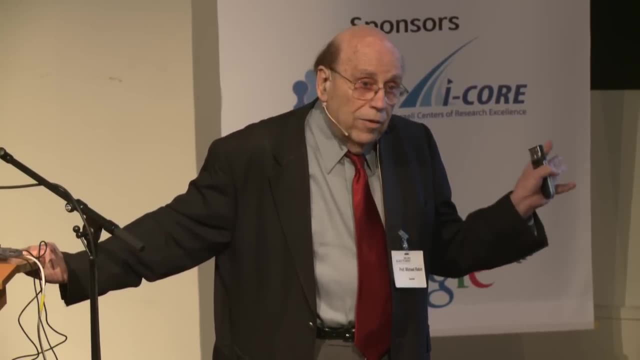 Now, I did not meet von Neumann, even though I had an opportunity to do so. I had a letter of introduction to him. I didn't want to bother him, But I spoke a lot to the people around him At Princeton, and also somebody who cooperated with him. 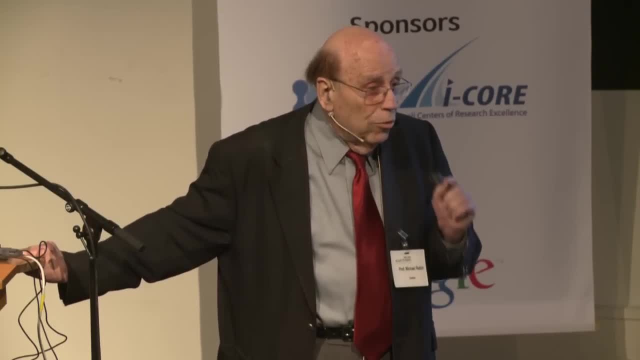 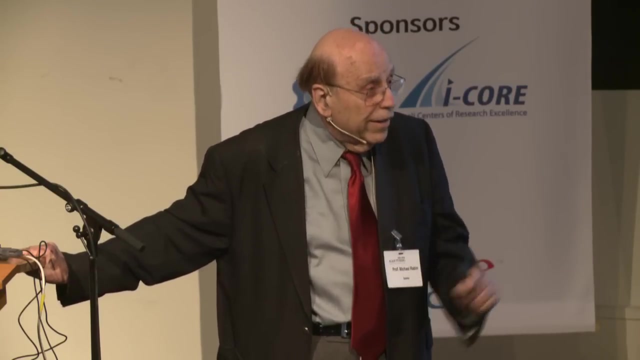 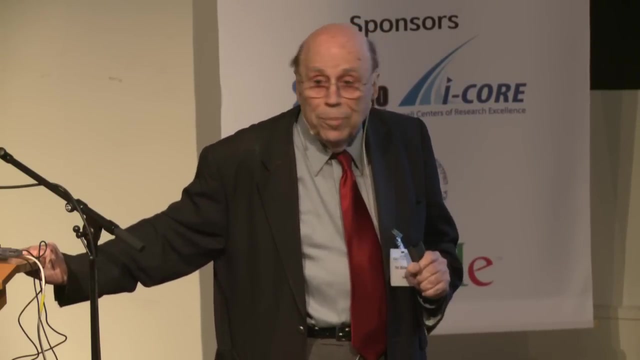 Burks And there is absolutely no doubt that von Neumann was deeply aware of Turing's work. Turing was at Princeton and there is absolutely no doubt that von Neumann was deeply aware, And he himself said, that those ideas of having a stored program and the instruction cycle and so on, all of that was revealed to him, to von Neumann, via Turing's basic paper. 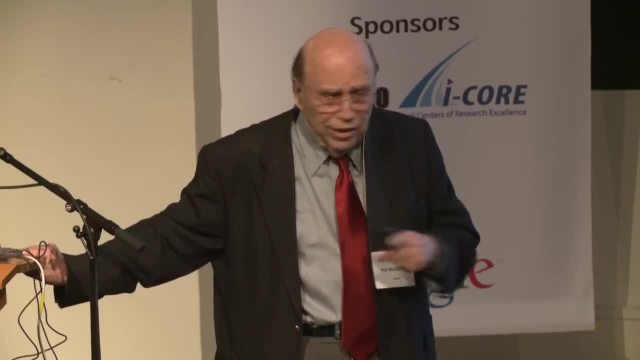 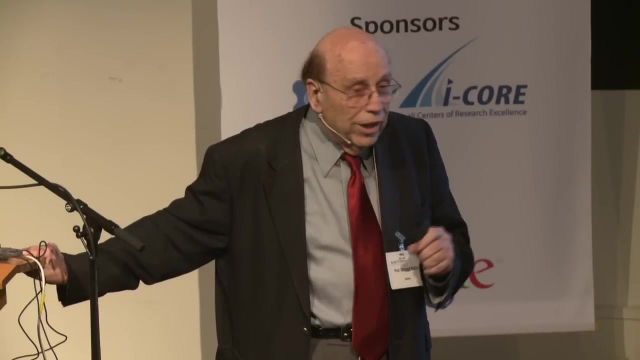 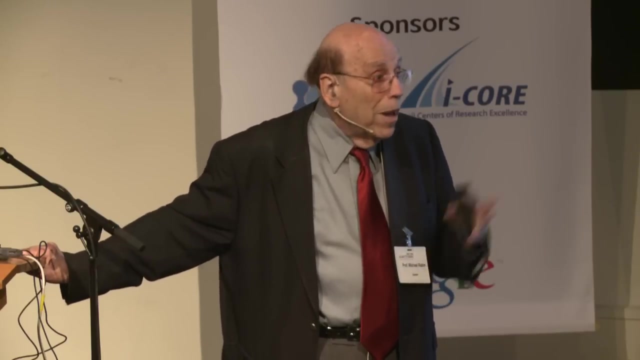 They spent together some time in Princeton for a couple of years, as was mentioned here by the introductory historical lecture. On the other hand, von Neumann was not only a wizard architect. The electrical engineers who worked with him said that when they had some circuit, they had to design some electronic circuit. they had to design and they couldn't really solve it. they would bring the problem to von Neumann, the mathematician, and he would settle it within about ten minutes. 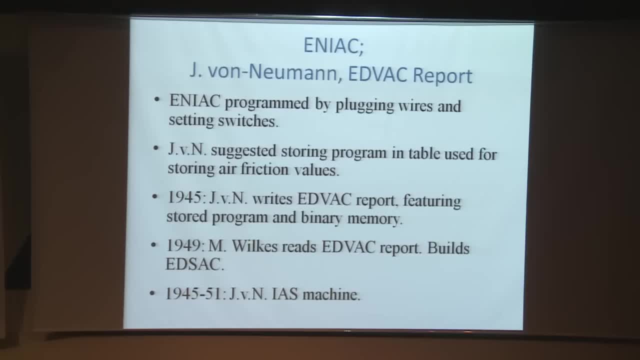 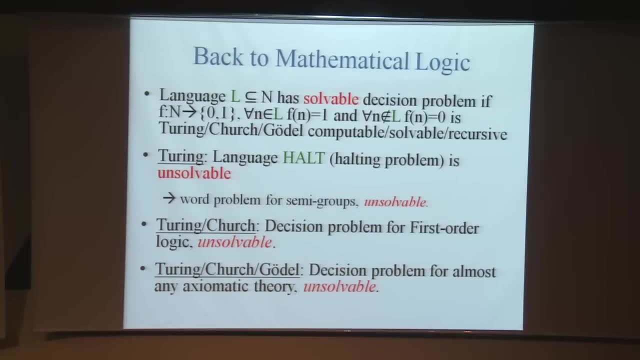 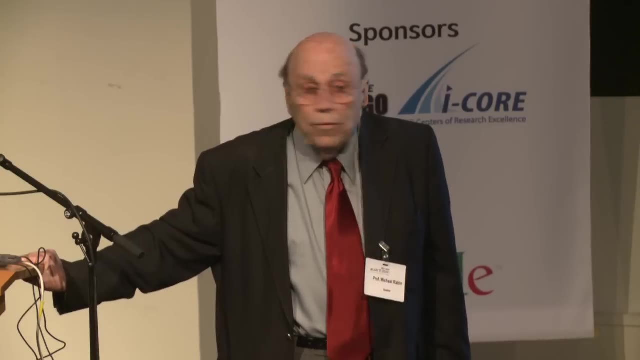 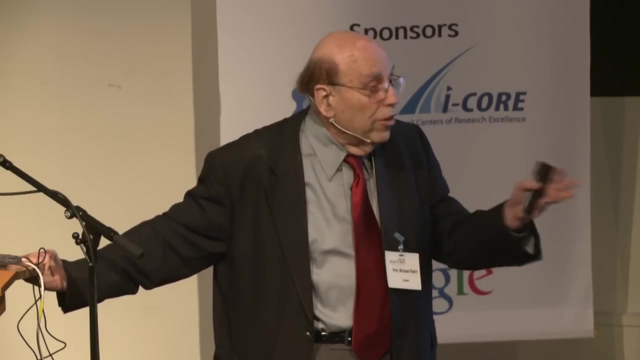 Okay, let that be an example to all of you, All of us here. So fine, Now we want to go back to mathematical logic. I said that the origins of this revolution was essentially in logic, in Hilbert's question, in the definition by logicians who wanted to answer the question what computability means. 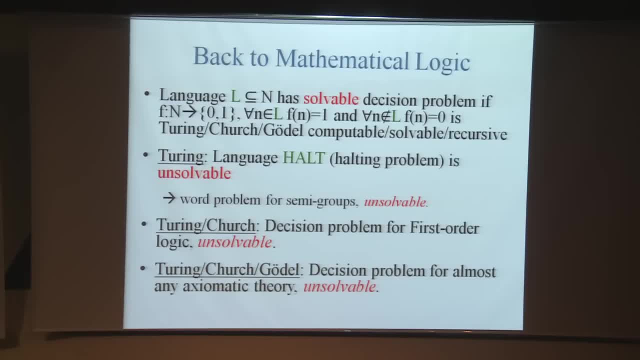 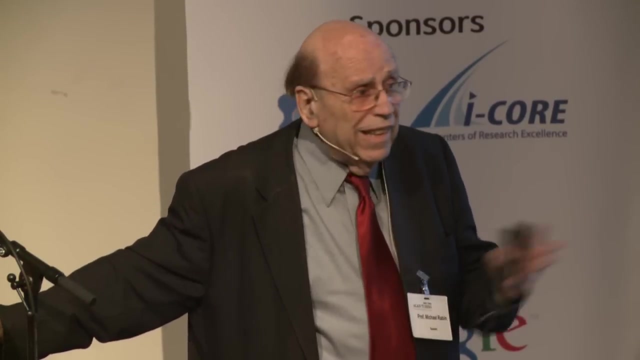 Okay, So now we want to see what these ideas did to logic itself. So N here, N is the set of all natural numbers, And if you consider natural numbers as being expressed in binary, so you essentially have the set of all worlds. 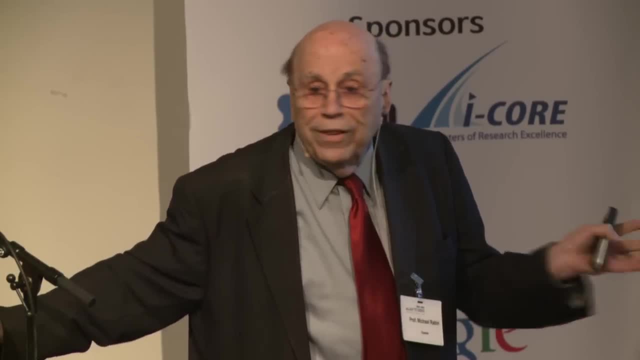 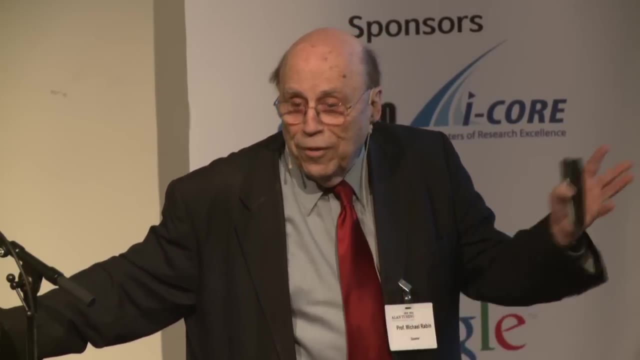 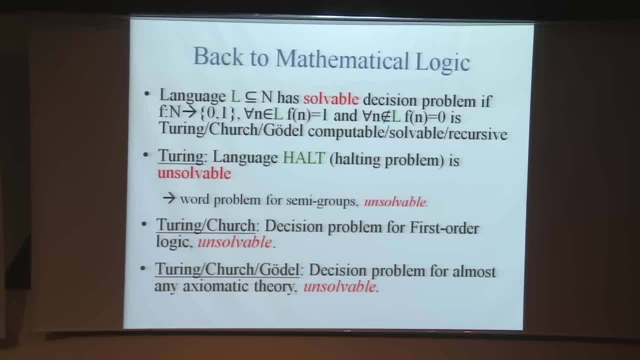 And a subset like that we call a language, We say it has. the language has a solvable decision problem if the characteristic function, the function F, from N into 0,, 1, which is 1 if N is in L and zero if n is not an l. 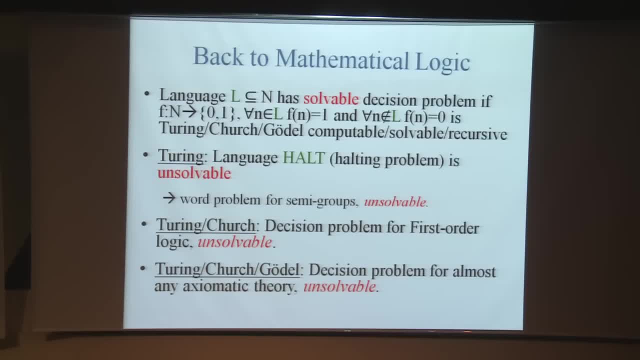 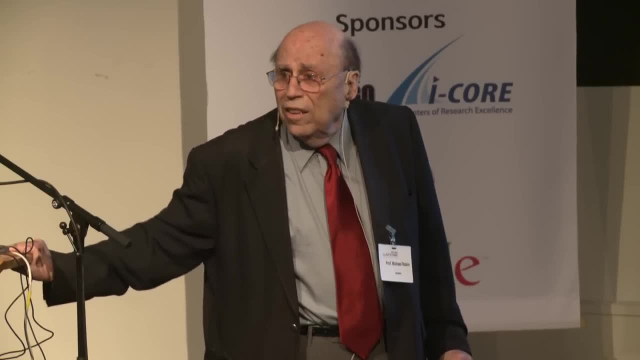 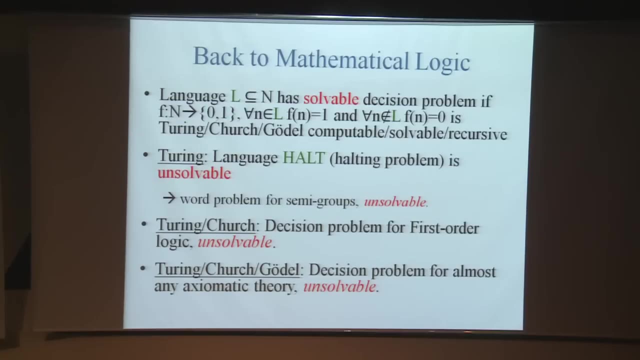 is Turing church girdle computable Also later on. the language instead, because of recursive functions, such a function is also called a recursive function. Now Turing has shown in the original paper that the language halt, namely the language meaning the set of binary sequences. 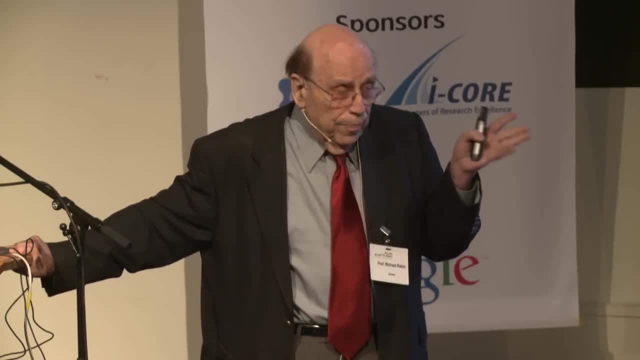 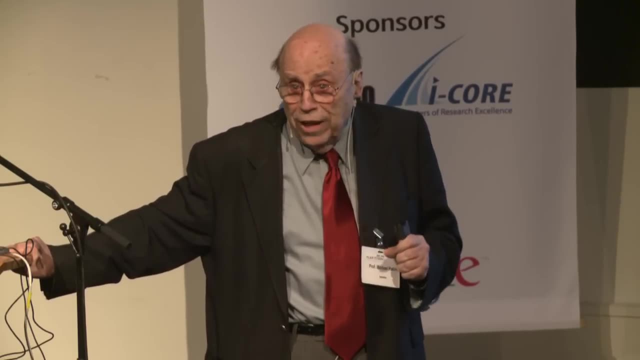 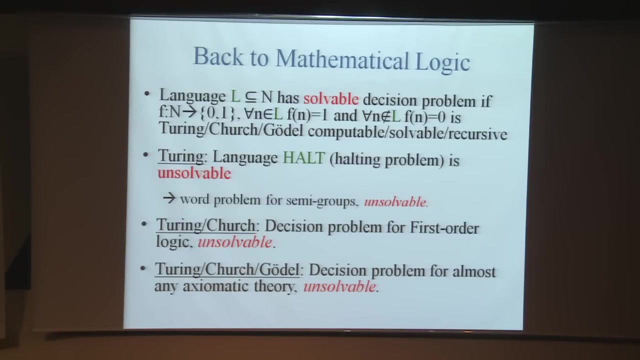 describing all computer programs that halt, that stop. let's say on the input zero that that language, meaning the halting problem, is unsolvable. This was the first indication and we are going to hear, I think, a little bit more about this. 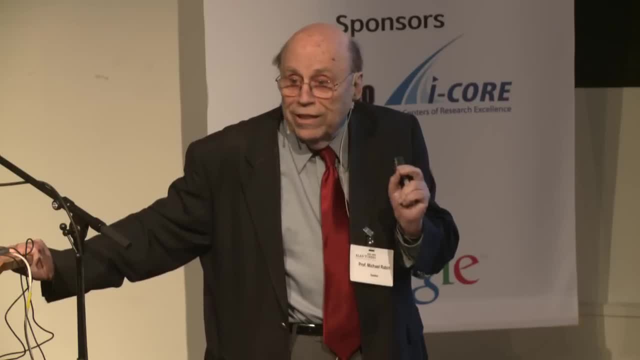 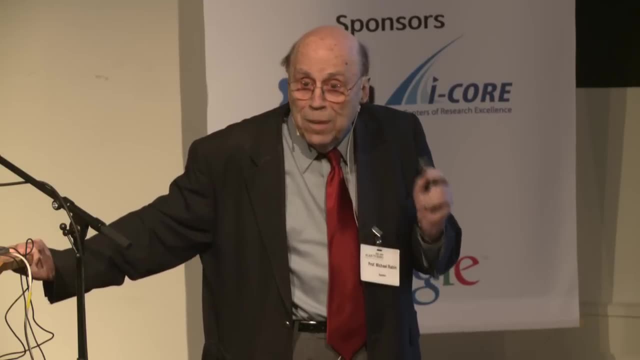 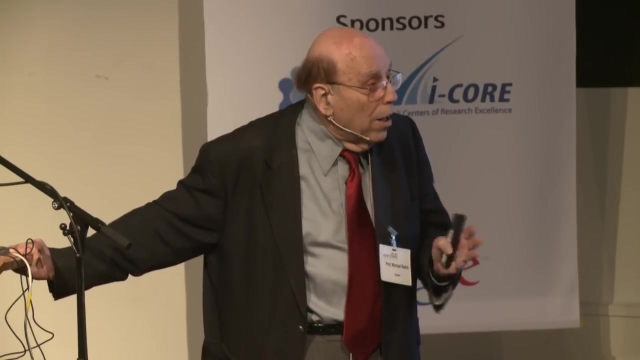 in a lecture about that, that programming languages are completely and their correctness is a completely non-trivial topic. Namely, there is no in general computable solution to say whether a program is correct, not even whether that program on a given input. 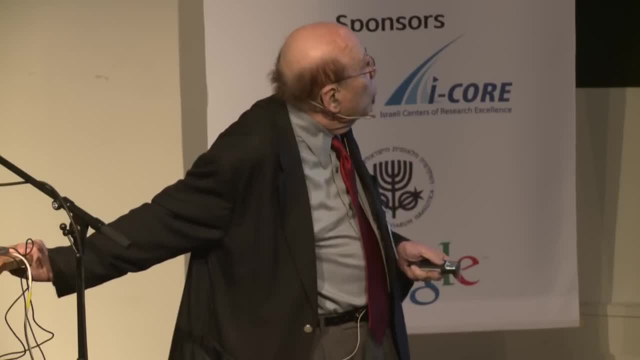 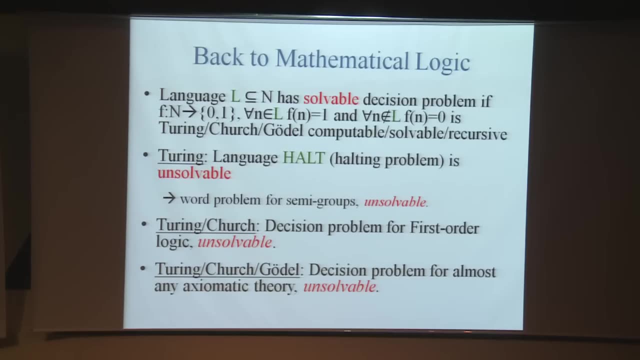 is going to stop and produce an output From that he derived and this is technical but very cute and I read all of that stuff and it made an enormous impression on me that the world problem for semi-groups, that problem is unsolvable. 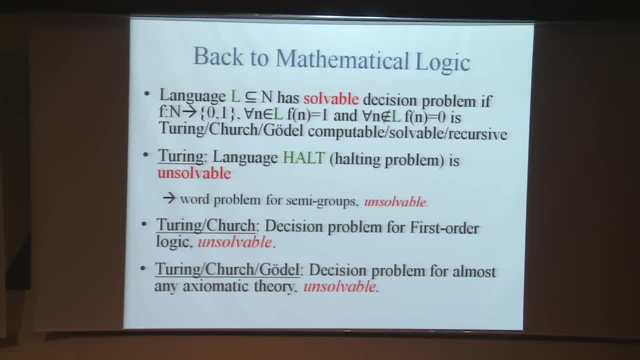 If you don't know what that means, it doesn't matter. Now, Turing and Church have shown that the decision problem for first-order logic, given a formula of first-order logic, the question whether that formula is a theorem- this is unsolvable. 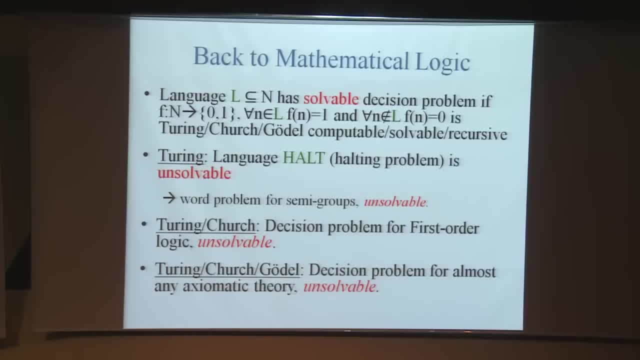 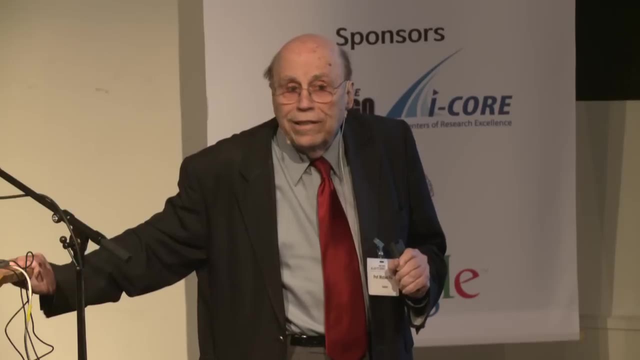 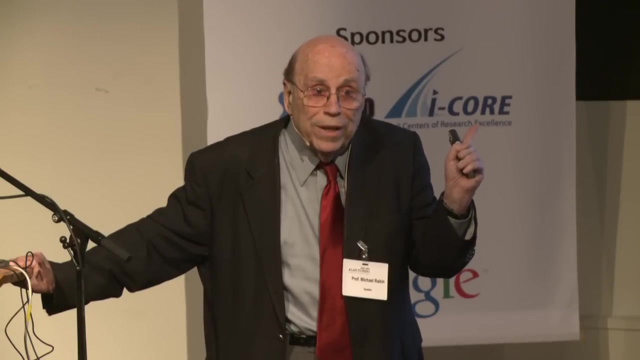 In a sense meaning that mathematics is not trivial. And it turned out that Turing Church, Gödel have shown that the decision problem for almost any axiomatic theory is unsolvable, To say for any axiomatic none. and I'm going to give a counter example in a moment. 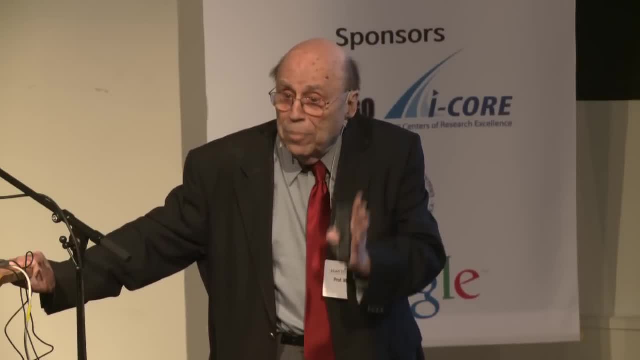 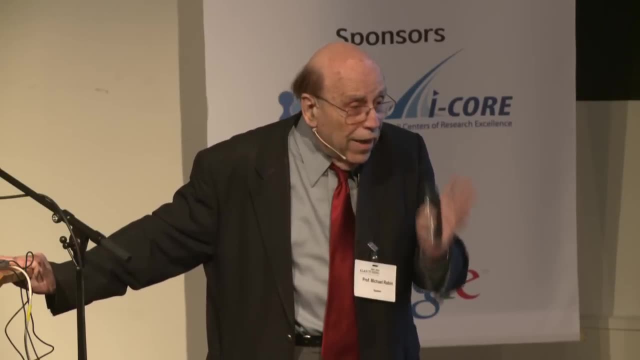 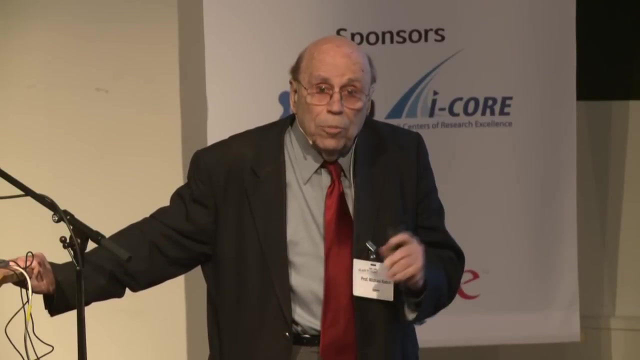 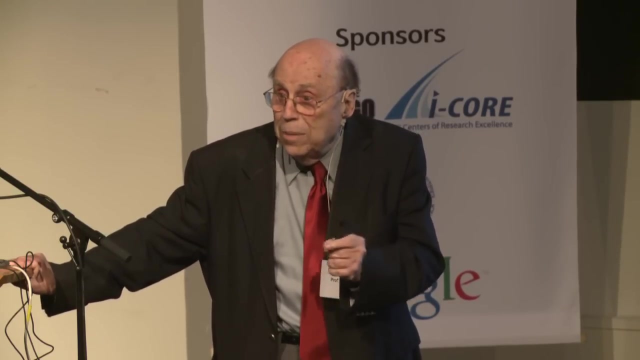 In particular, if we take the natural numbers with addition and multiplication and we talk about the question which sentences there are true or not, or which sentences are theorems of what is called Peano arithmetic, that set is not recursive. You cannot build any machine. 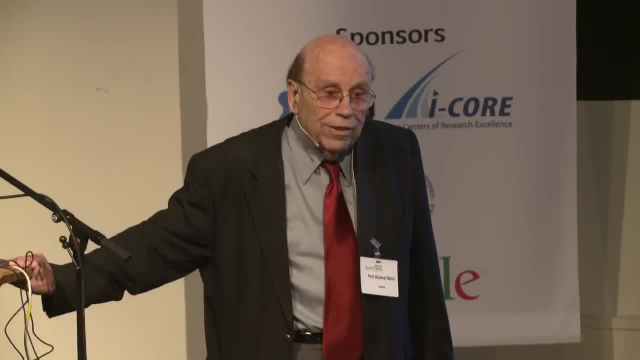 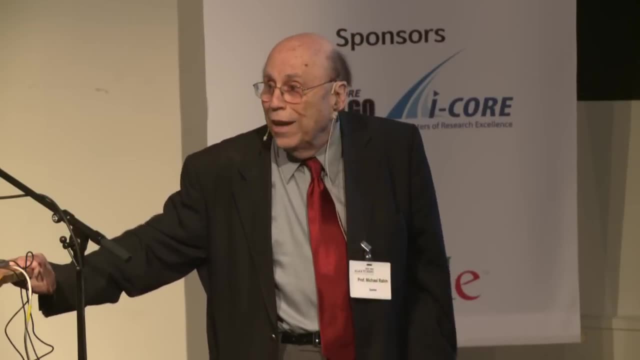 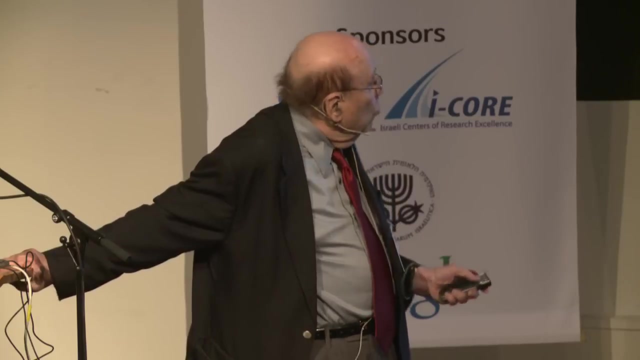 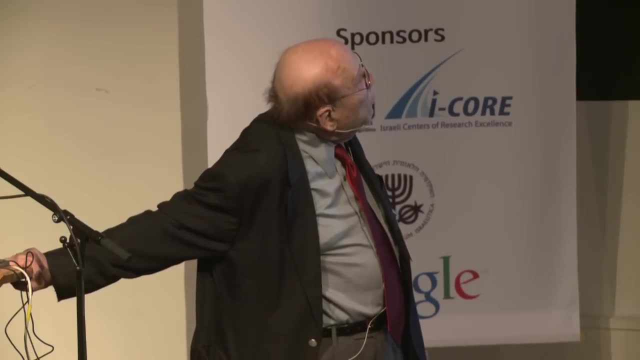 that is going to automatically answer those questions. So that was a sort of a complete death sentence to the Hilbert program of finding an algorithmic solution to the question: what is a theorem and what isn't? Now we want to go to unsolvability, to complexity. 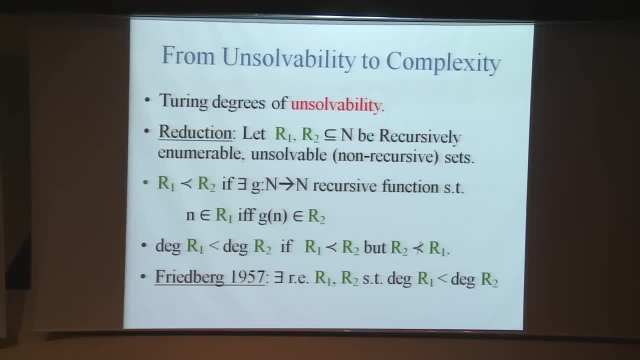 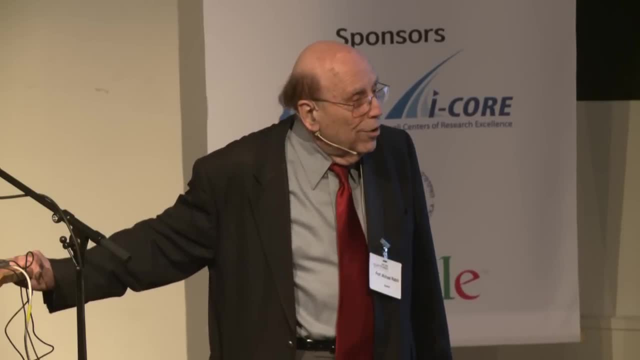 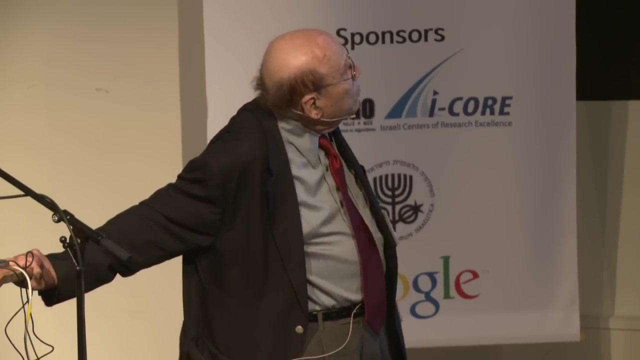 So I'll arrive at complexity for a moment, and I'm going to do- because my boss here is going to tell me very soon that I don't have too much time- I'm going to sort of miss, I'm going to skip that. 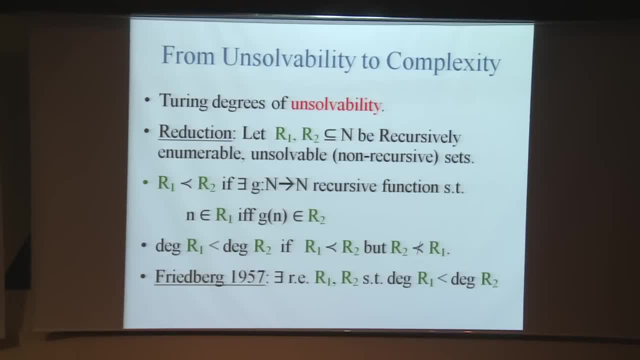 But essentially- and you'll have to follow very quickly this suppose we have recursively enumerable but unsolvable non-recursive sets. It turns out that Turing already suggested a hierarchy of unsolvability And he raised the question whether there are really 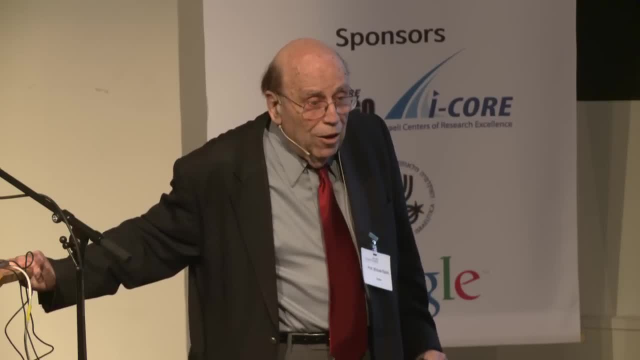 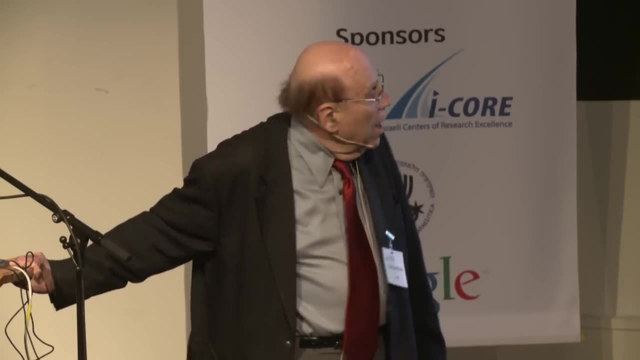 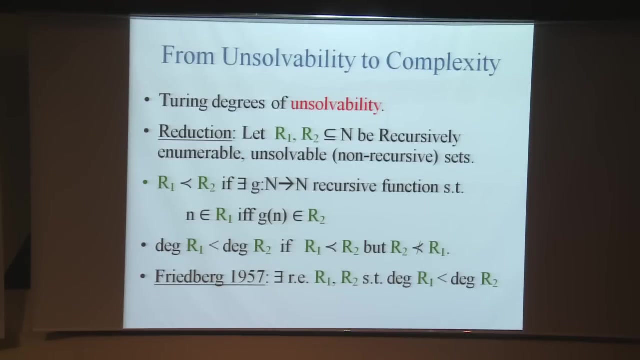 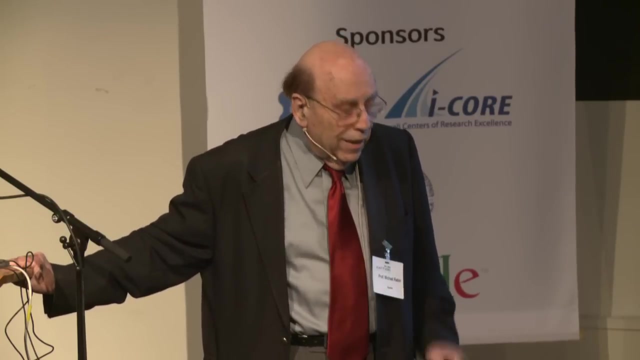 unsolvable problems, unsolvable of different complexity, of non-computability. And that question was answered by Fischer, by Friedberg, who showed that, in fact, the degree, in the Turing sense, the degrees, form a certain hierarchy and that there is a whole hierarchy of unsolvability. 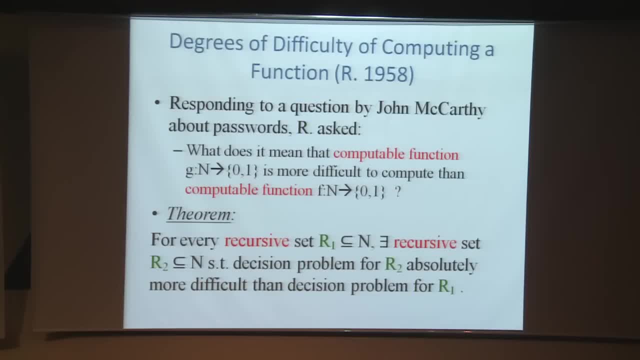 Now the next step: from those degrees of unsolvability we go to what I call the 1958 degrees of difficulty of computing functions, And now of course this is called complexity. I was visiting IBM in 1958,. 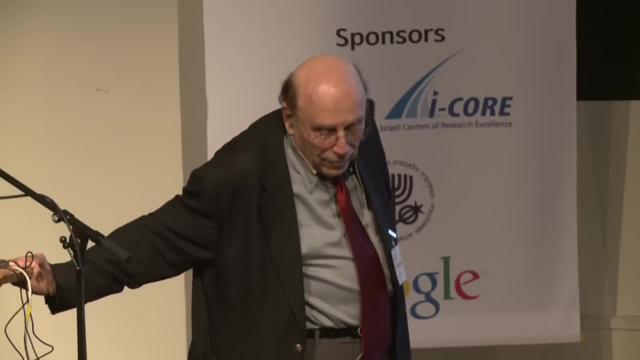 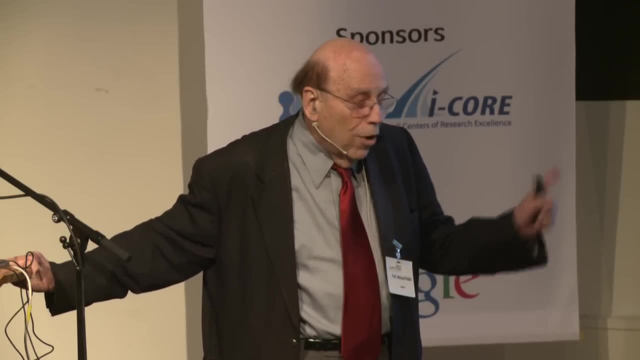 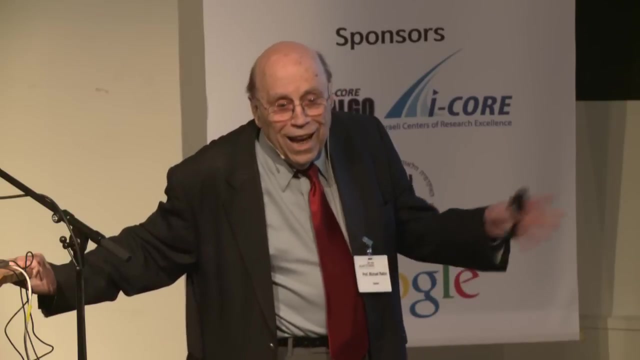 before they had the research center they were located in the place called the Lamb estate, Very appropriately. before they moved in and before they went to work And before I came to visit there, it was an insane asylum, But then we guys were sitting guys. there were almost no women. 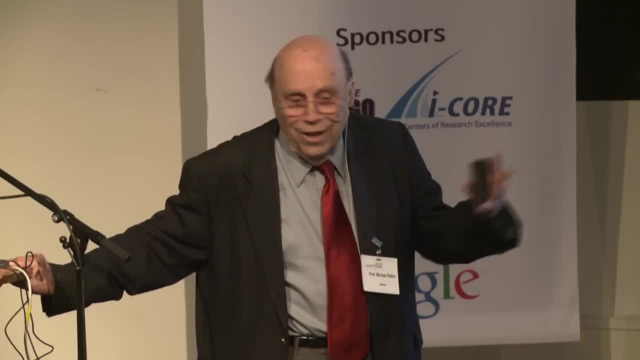 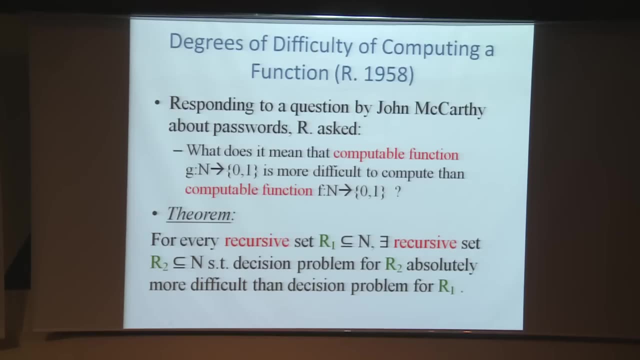 We were sitting there and working essentially on the early steps of what is now computer science. So there was a question by John McCarthy post to me about passwords. I don't have time, It's a lovely question. So it raised in me the question: what does it mean that for computable functions, for 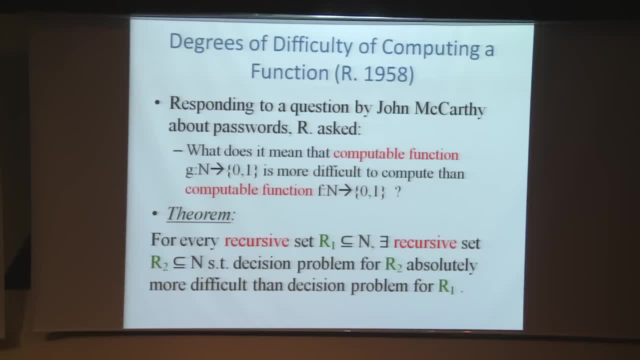 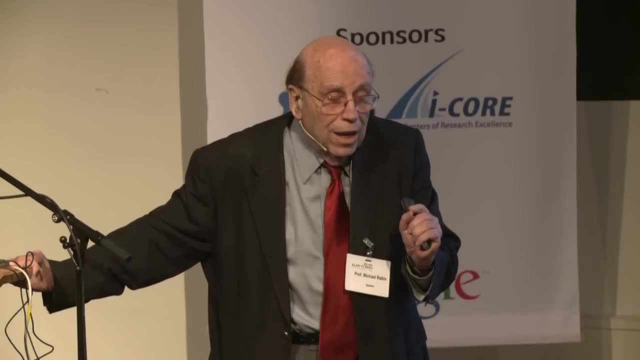 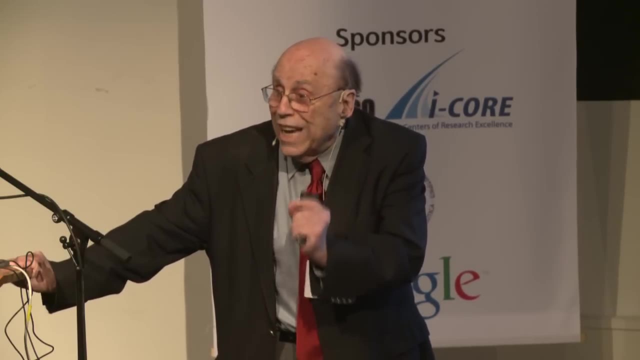 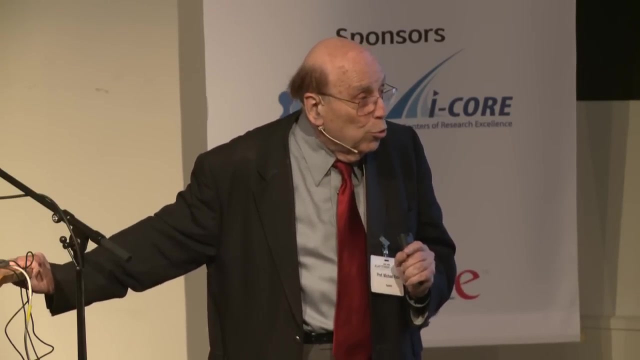 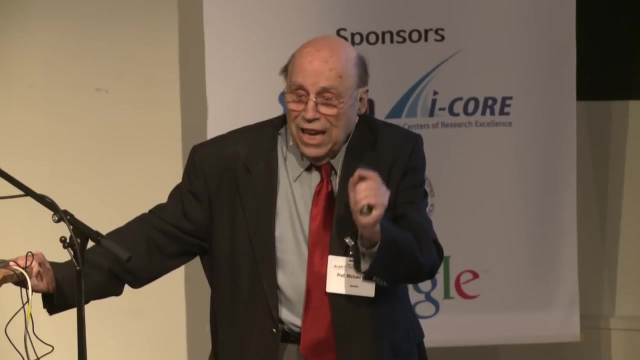 solvable problems. what does it mean to say that? one solvable in the Turing sense problem? there is another solvable problem which is absolutely harder. In other words, they are both solvable And hence, from Turing's point of view, trivial problems. still, there is a concept of what 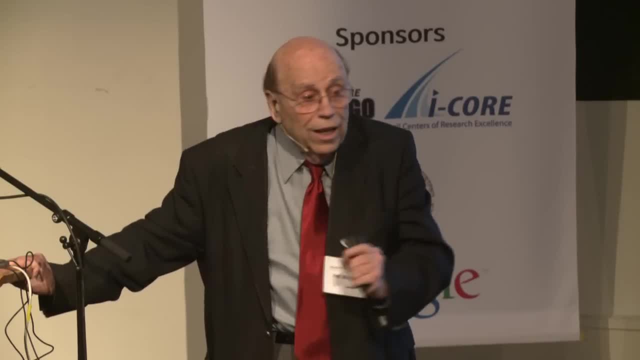 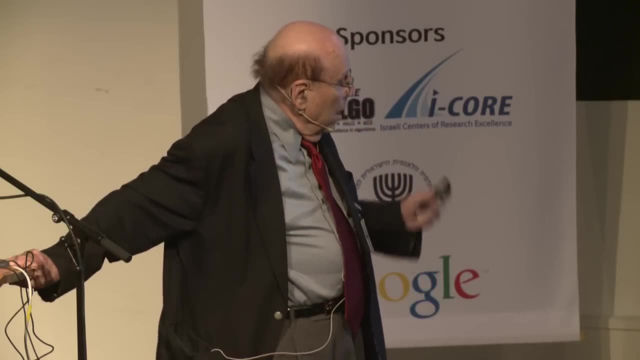 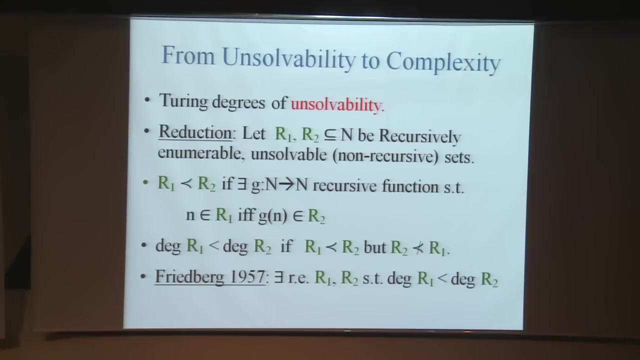 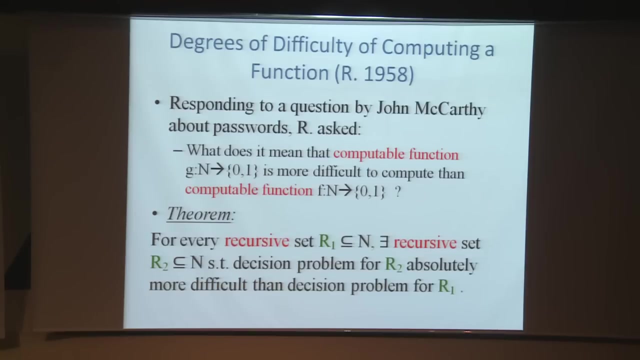 I call degree of difficulty and now it's called complexity, where one problem is absolutely more difficult than another problem, And I proved a theorem that, in a very strong sense, for every recursive meaning solvable There is another solvable problem, such that the decision problem for the second one is 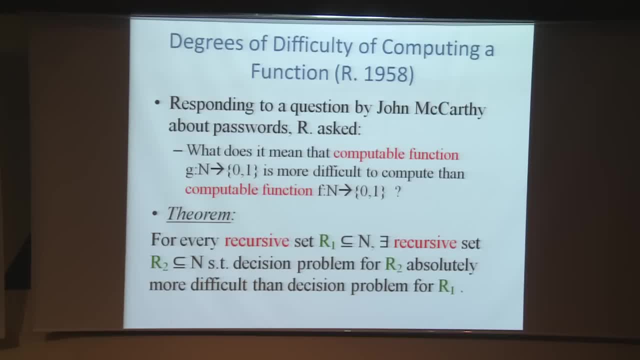 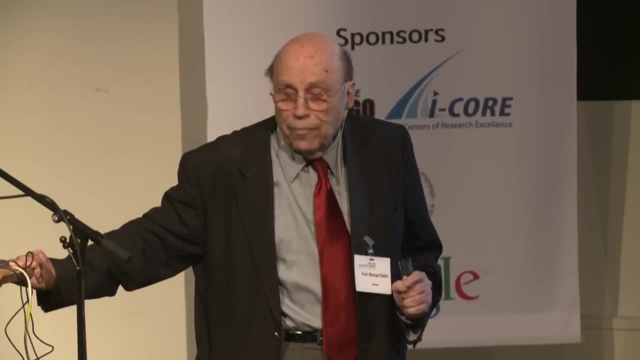 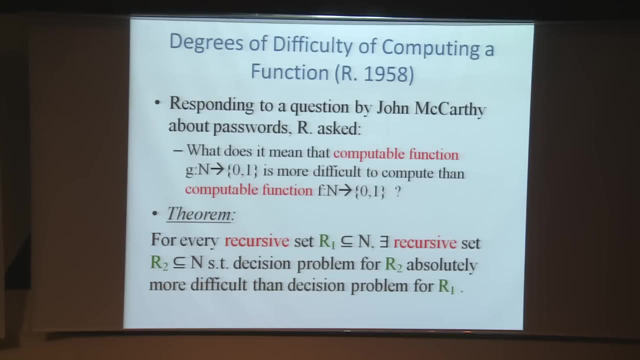 absolutely more difficult than the solvable decision problem for the first, So it is absolutely more complex. I can't go into the formal definitions anyway. If I would have done it, you would have forgotten it the minute you walk out of this hall. 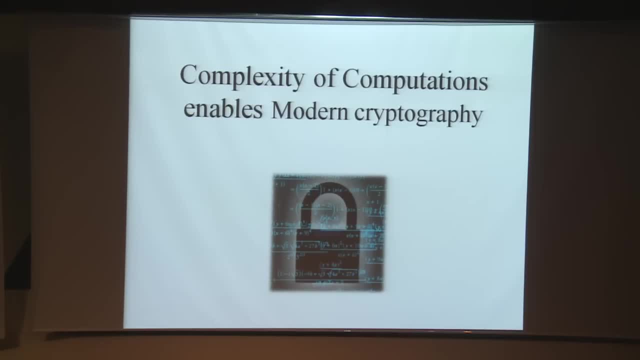 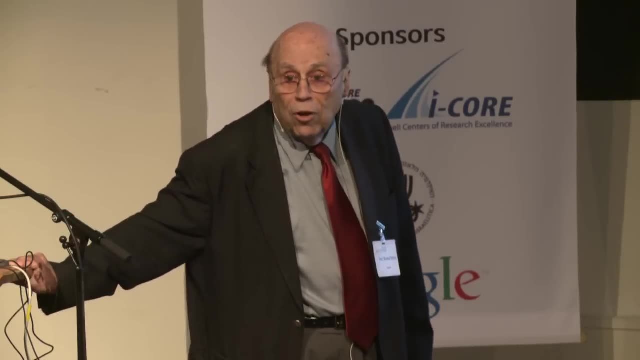 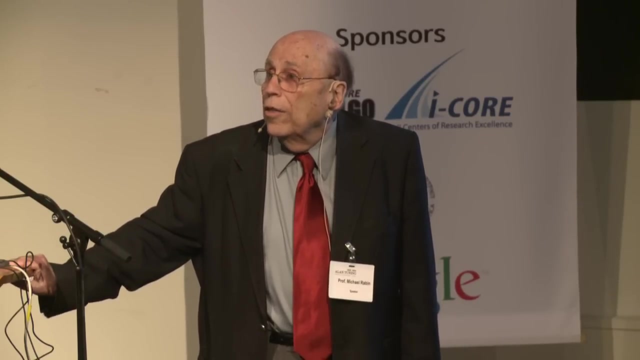 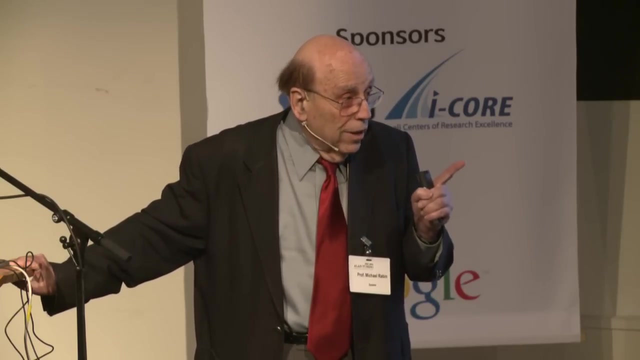 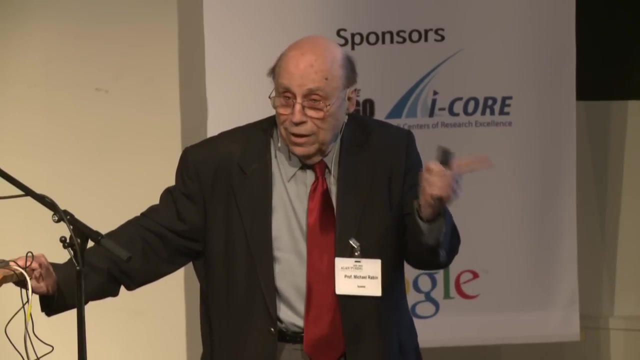 Now the concepts. complexity of computations is what enables modern cryptography. Modern cryptography is based on the proposition, as yet open, that there are functions, namely the encryption, which are easy to compute, whereas the inverse, namely the decryption, is hard. If that assumption turns out to be false- and we don't as yet know, there is no proof- 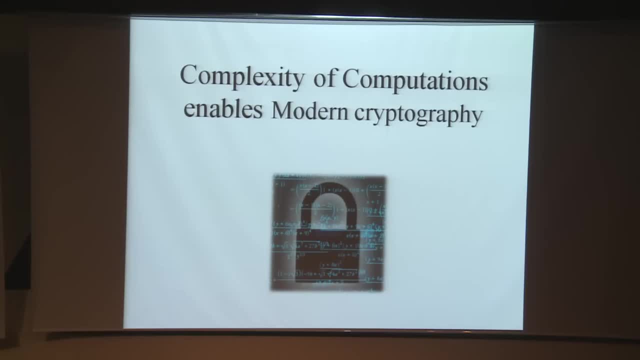 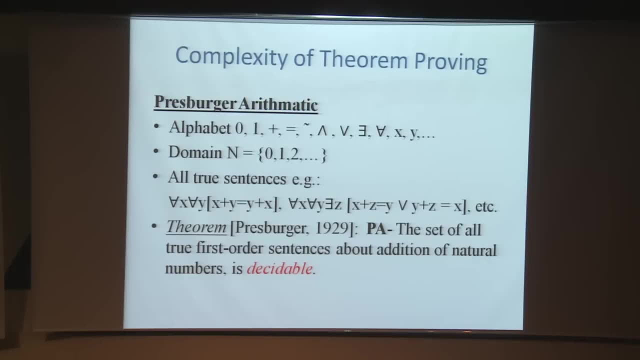 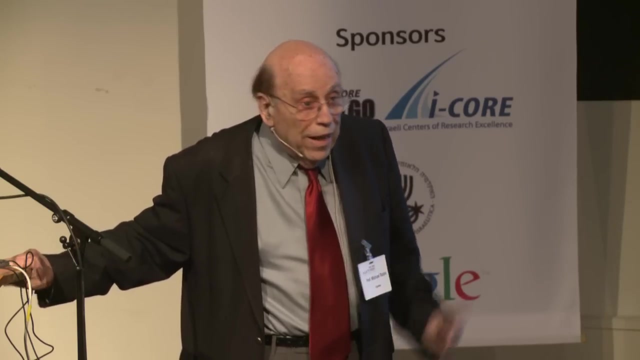 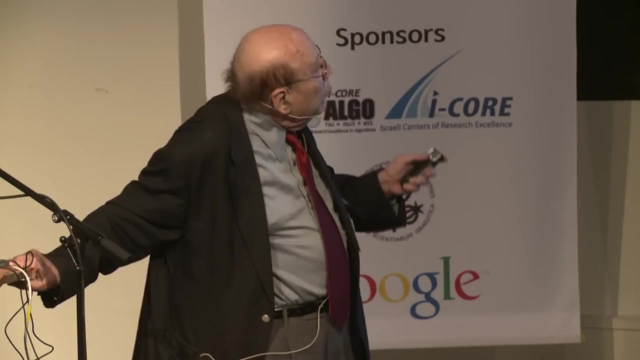 that that actually exists. if that turns out to be false, then modern cryptography is going to collapse. Now let us go back to theorem proving. There is a segment of the theory of addition and multiplication of natural numbers, that theory being absolutely undecidable in the Turing sense. namely, Pressburger, in 1929, considered: 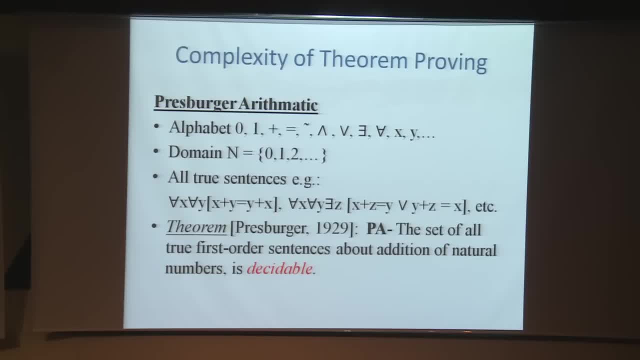 the natural numbers. So To get the formal language you have this alphabet. the domain are the natural integers, the operation is addition and examples of true sentences are: for all x and for all y. x plus y is equal to y plus x, which means addition is commutative, addition of natural. 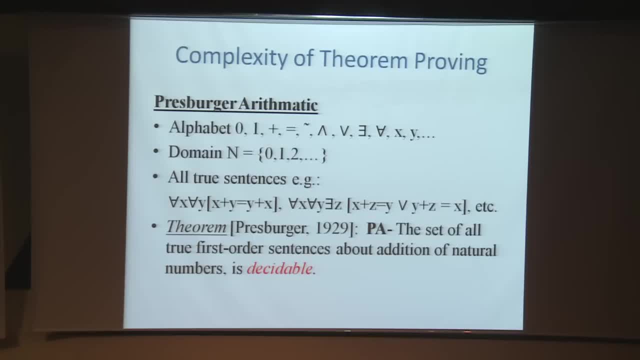 numbers. For all x and for all y there exists a z. Remember that The numbers are 0,, 1,, 2, they are the non-negative integers, So that x plus z is y or y plus z is x. 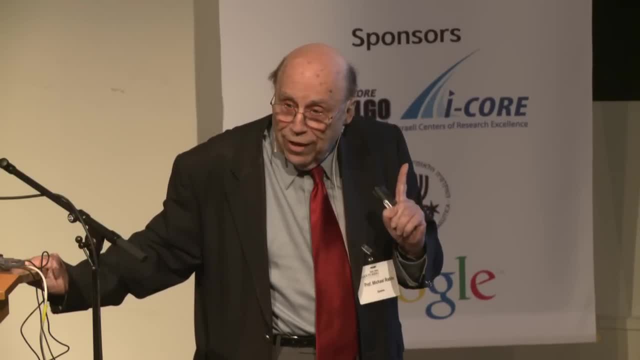 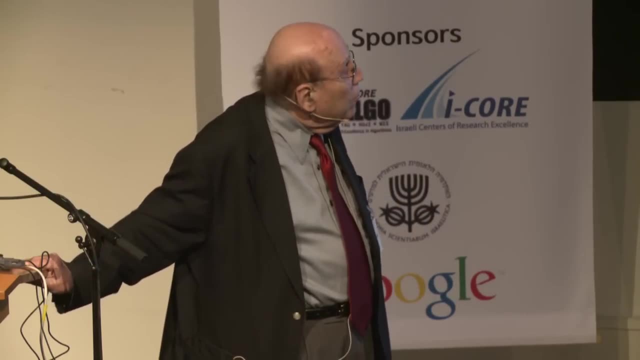 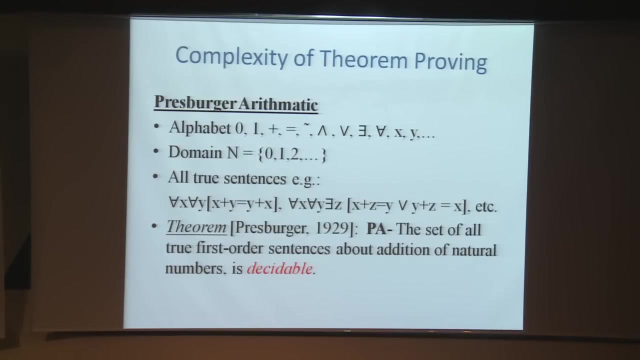 In other words that there is an ordering there, that they are actually linearly ordered. by this relationship, And Pressburger in 1929 has proved that the set of all true first order sentences about addition of natural numbers is decidable. There is a decidable. 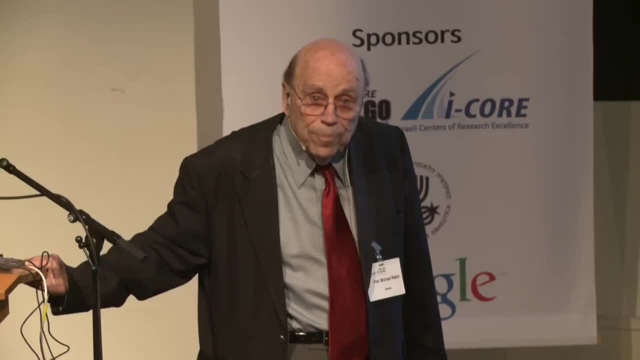 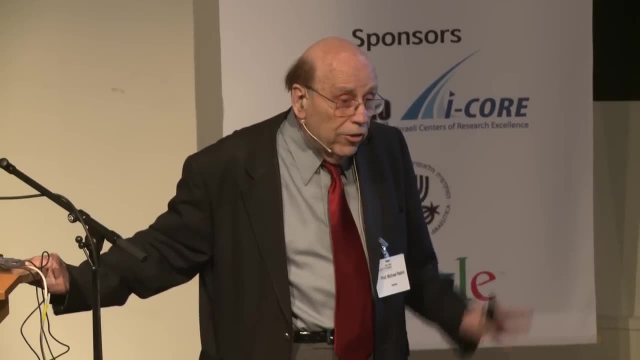 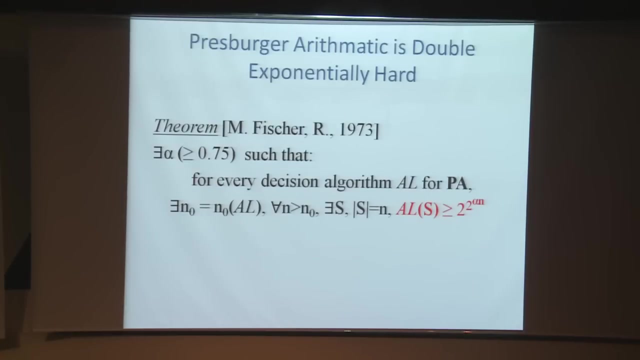 There is a decision procedure for that. In fact, people in program verification were very interested. there are various applications for that. Okay, it's decidable Now. Michael Fisher and R in 1973 have shown that there exists an alpha. 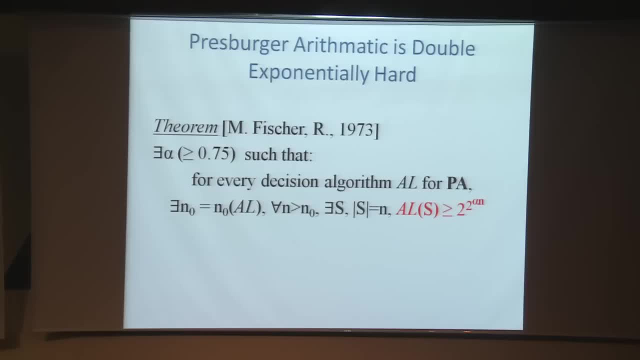 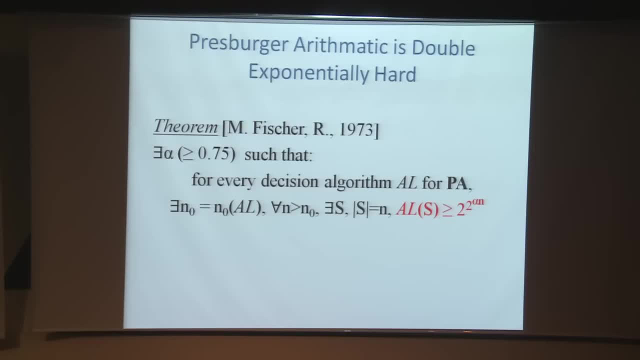 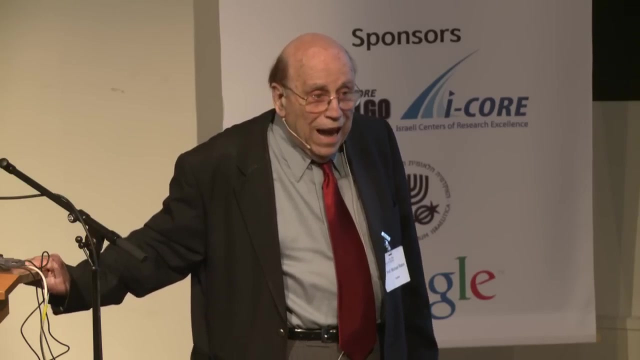 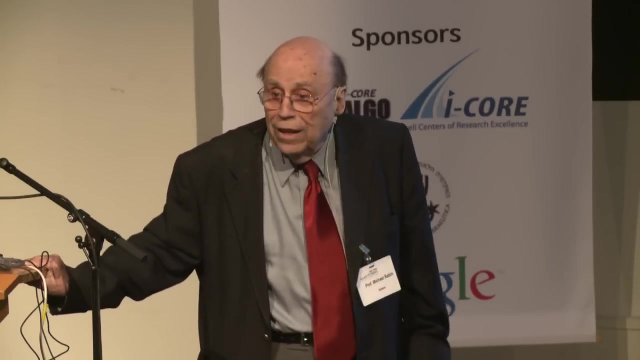 is an n0 dependent on the algorithm, So that for every n greater than n0, there exists a sentence about addition of length n, So that the algorithm applied to that s- that's shocking- takes more than two to the two, to the alpha times: n steps to give you the answer. 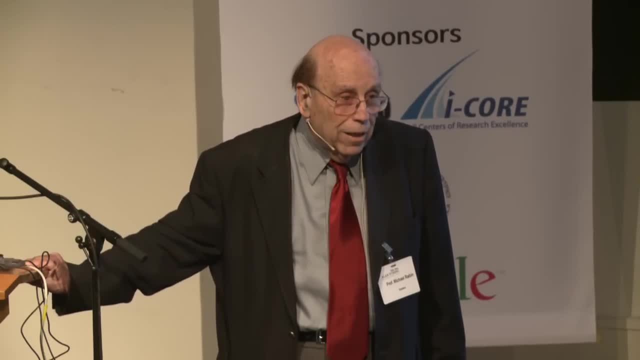 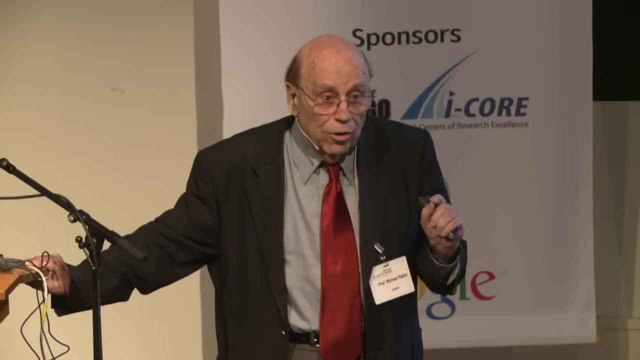 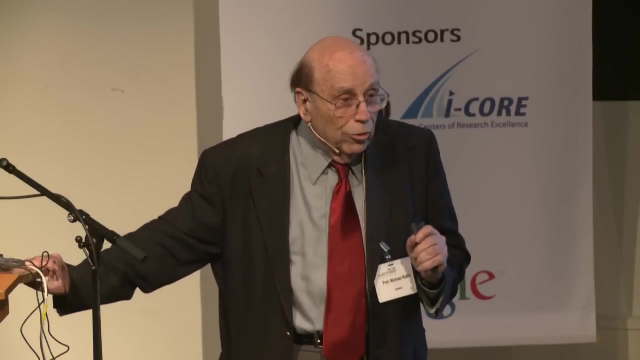 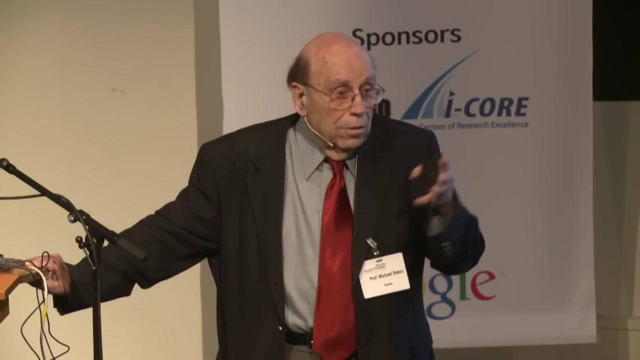 It's doubly exponential, absolutely devastating. The n0 is not very large. The n0 is essentially the size of the algorithm. So that means Okay. So that means that if you have an algorithm which takes a thousand symbols to describe, there are going to be sentences of length for every n greater than 1,000.. 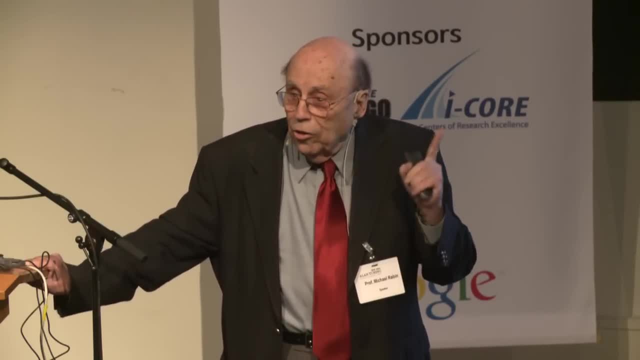 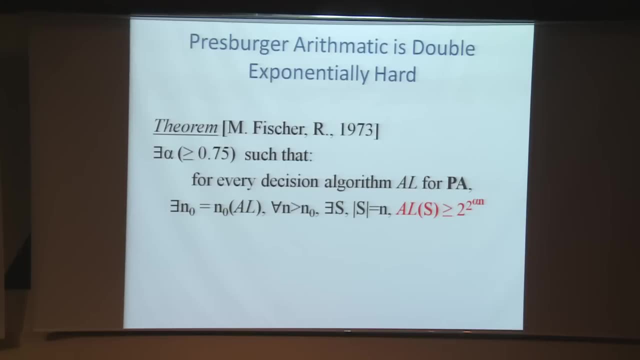 So let's say, of length, 1,000. So that applying that algorithm to get the correct answer will take two to the two to the seven hundred and fifty steps to give you the answer. Absolutely devastating, Good or bad depending where you look at it. 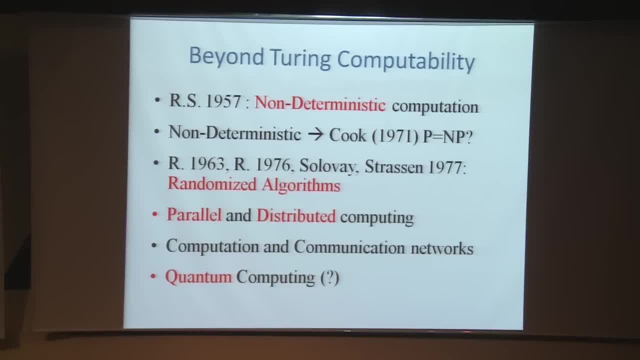 Now beyond Turing computability. So R and Scott in 57 introduced the notion of nondeterministic computations. 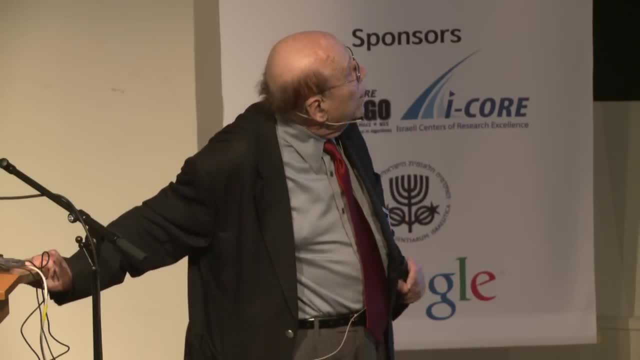 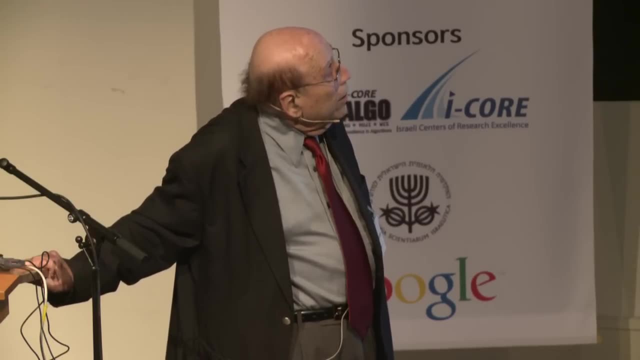 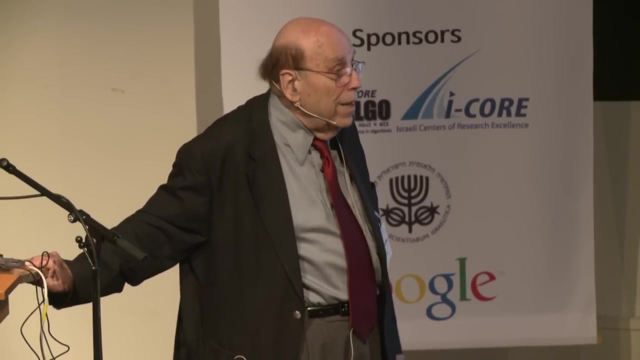 but they are also sort of extensions of the ideas of Turing non-deterministic led. I mean that concept was used by cook in 1971 to pose the classical question whether p equals to NP. If you don't know what that is, go and google it. 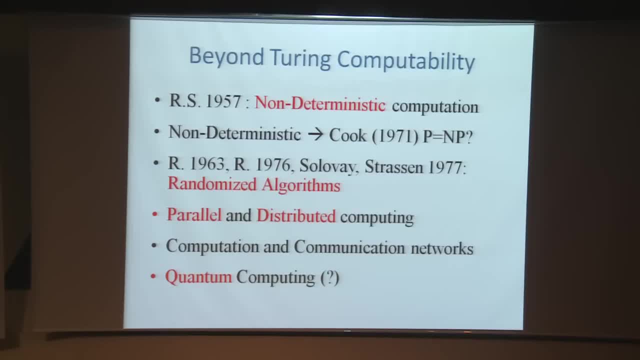 You will really learn something, and that question, by the way, is essential to the question whether 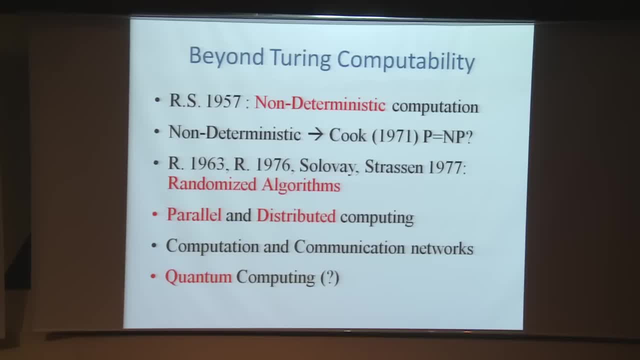 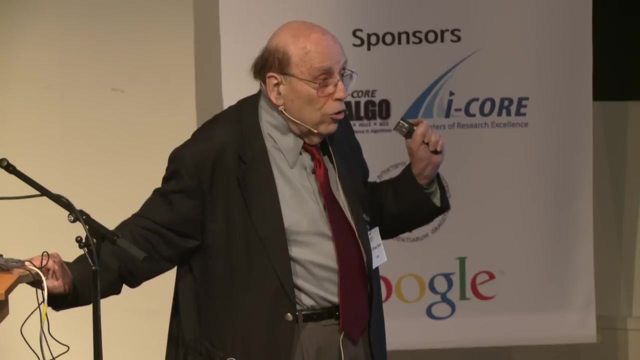 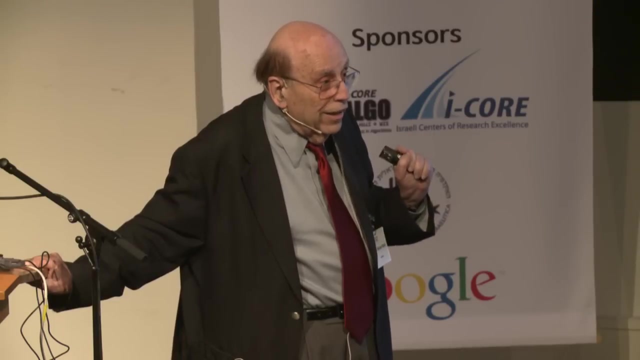 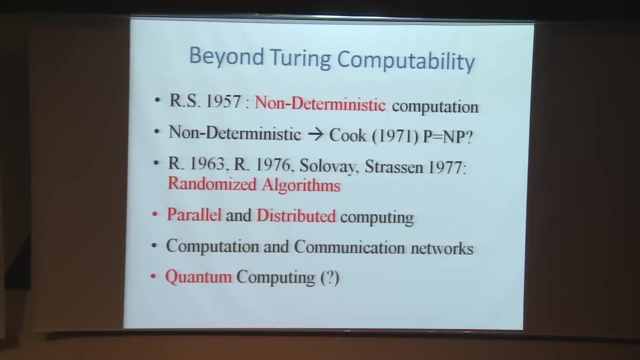 cryptographic algorithms are really, really skew. then in 1963 I had an extension of non-deterministic, namely probabilistic, automata where you use coin tossing and that turns out that this simplifies automata in certain cases greatly. and then in 1976 and Solovey Strassen 1977 had sort of the 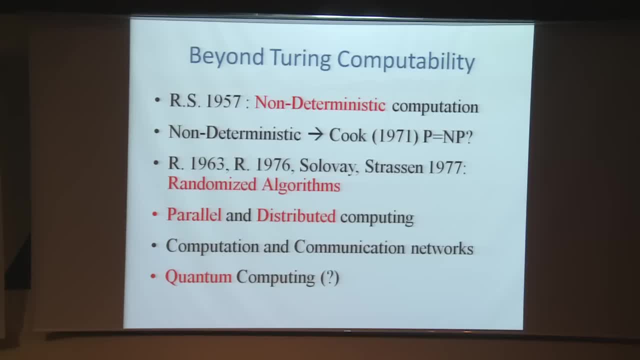 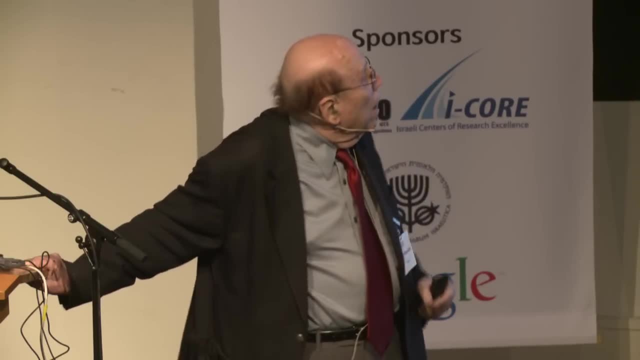 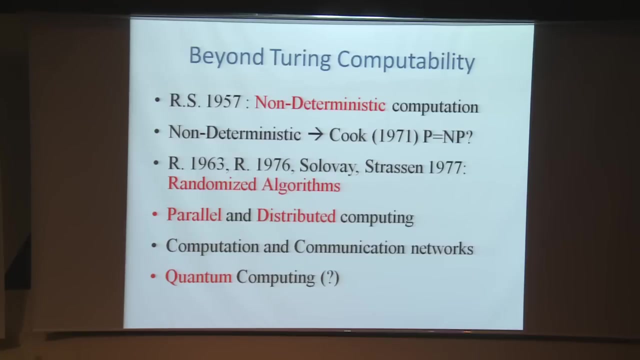 general idea of randomized algorithms, where you use coin tossing in order to speed up computations, and then, of course, parallel and distributed computing came in, and then, of course, communications and computations came in. and then, of course, communications and computations came in, computation networks and quantum computing came. I don't think Turing thought. 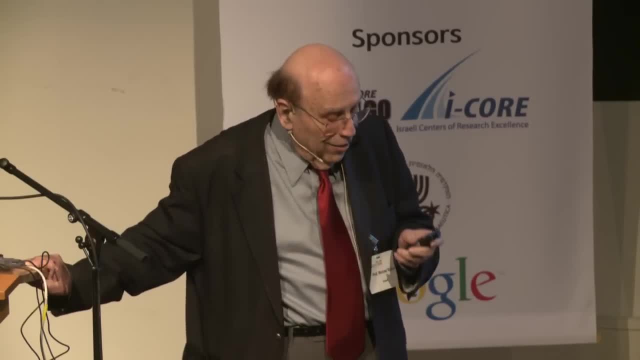 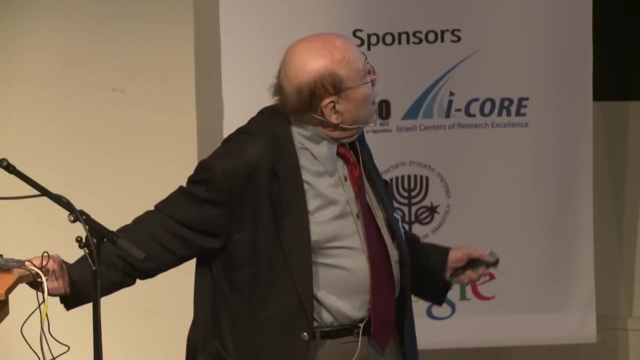 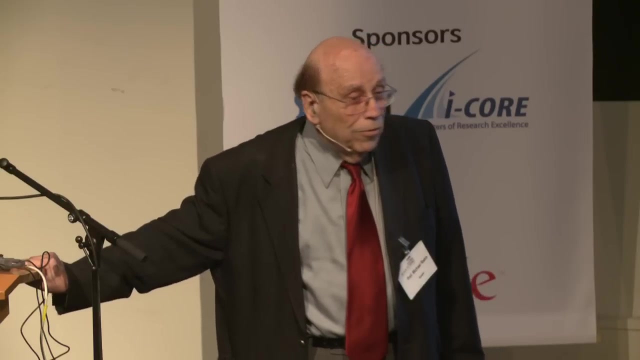 of that. I put a question mark there because we don't yet have the verdict whether that is feasible or not. and now I want to come to the future and I'm going to give two examples of what I think, and I had discussions here with Al Spector. 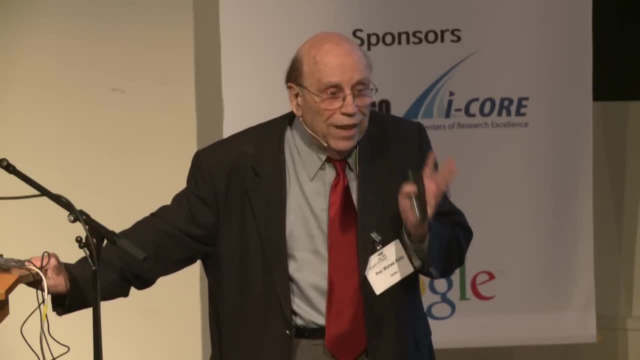 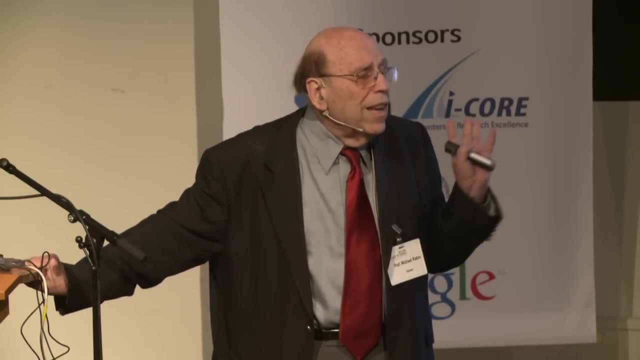 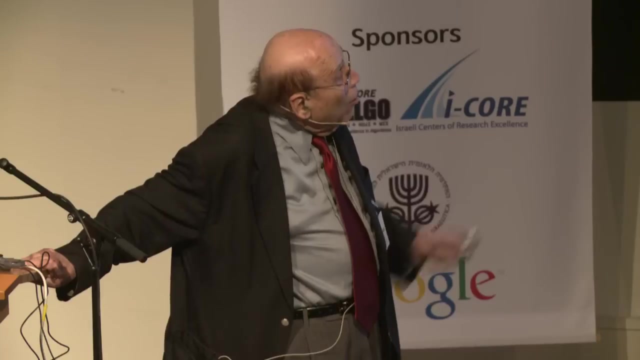 you know the next, some two at least, of the next very big things that will come about by use of that technology. I'm skipping Facebook, things like that. they are very important and created revolutions and so on. but university education now. I taught the course at Columbia which was recorded, and then 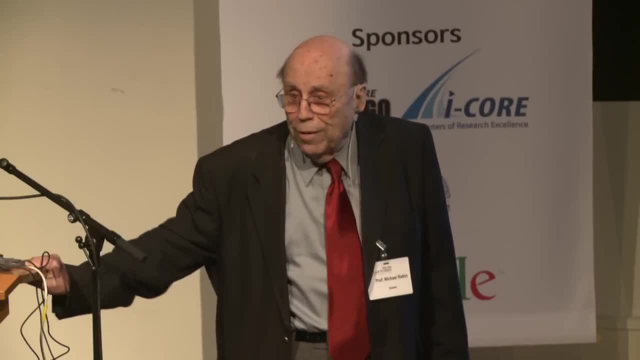 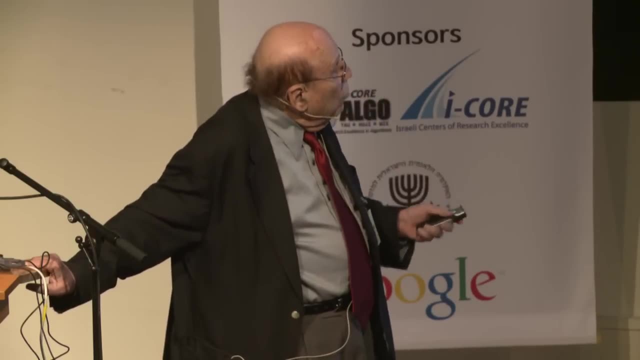 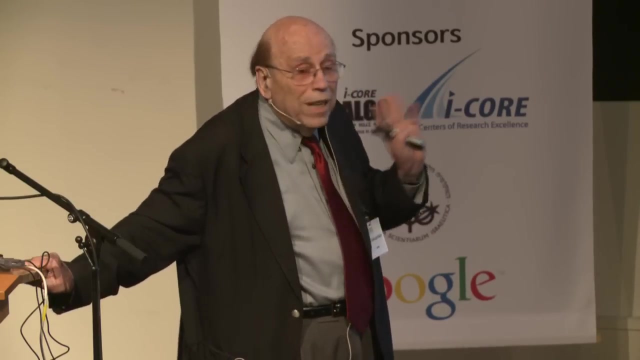 distributed to third-party universities and then I had discussions with the early 30 or 40 people all over the world, but that was done in a very primitive way. I envision that you're going to have a classroom, say at Stanford. Stanford is entering into this, but in that classroom and I'm only going 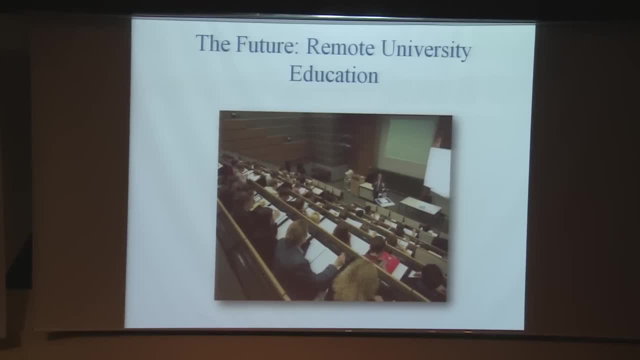 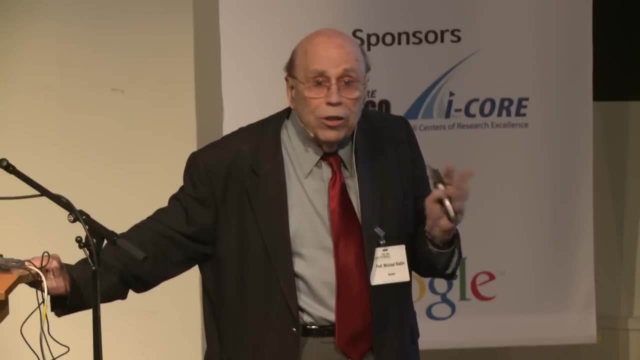 to give you, you know, the bad outline in that classroom while it is being taught here. like this: they are going to be six or seven cameras controlled in search of some way and those cameras are going. one is going to focus on the speaker, another one on the speaker and the board, the blackboard, whiteboard. another one is 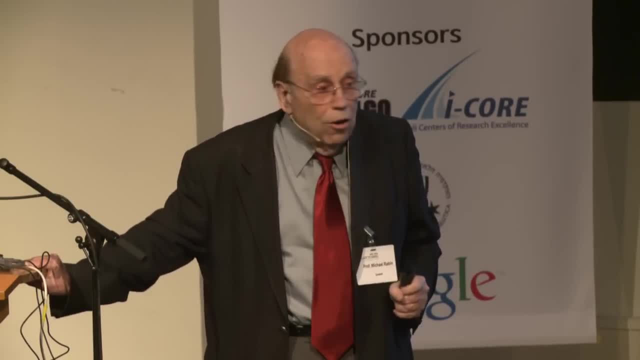 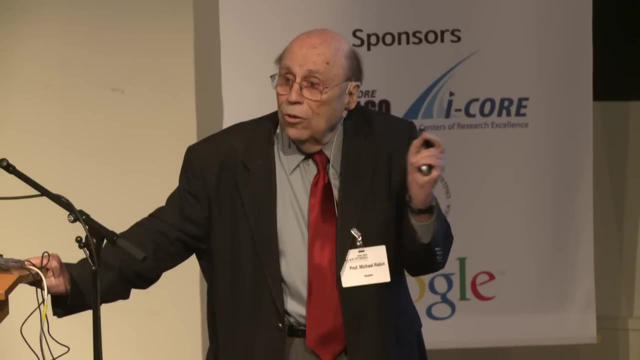 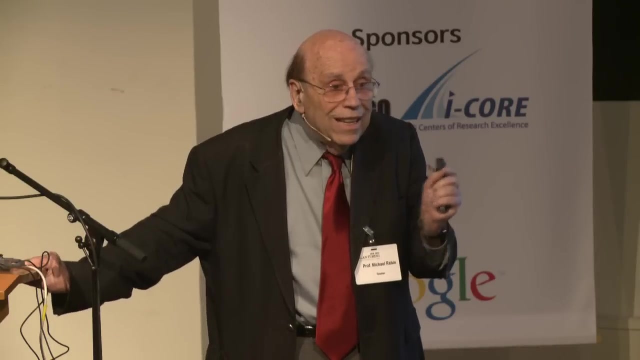 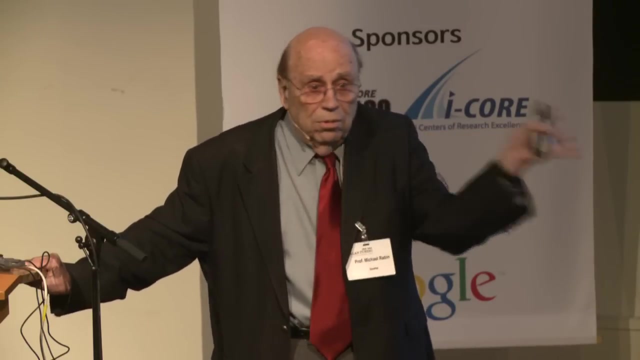 going to focus on various people in the audience and so on. all of that will be recorded and then somebody who is not fortunate enough to be at Stanford within that lecture is going to look at it and he is going to control also the output of the cameras. he is going not in real time while the lecture is going on. 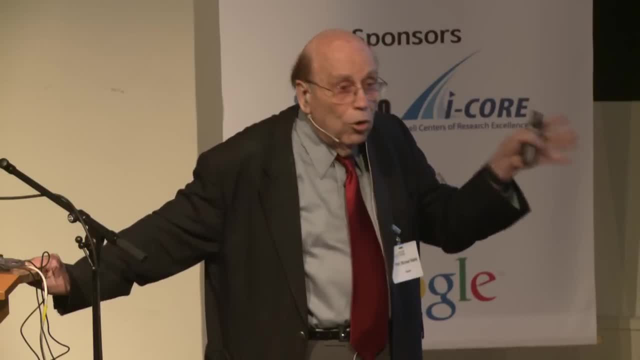 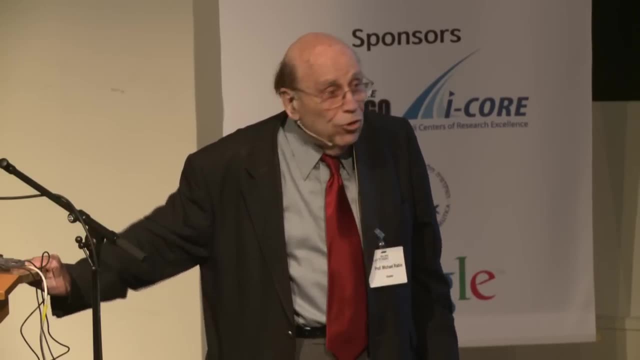 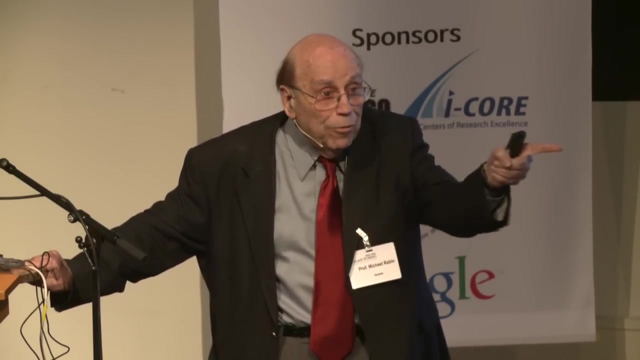 not in real time. he's going to see the board. he's going to see the speaker. he's going to see the board expression on some of the people in the audience. somebody asks a question that he can choose a camera focusing on the person who asked the question, and so 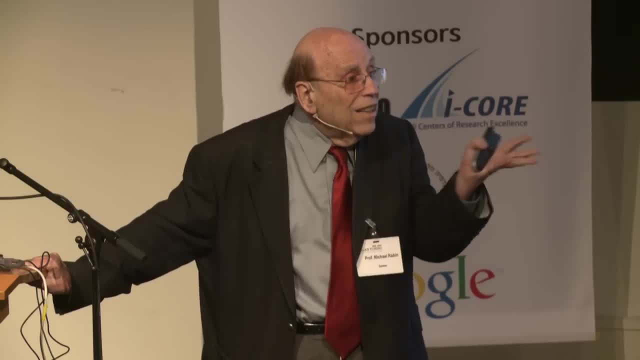 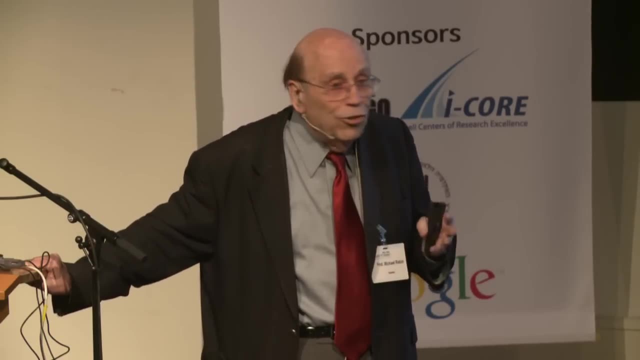 on, and this is going to give a hundred thousand people all over the world a feeling of again using a cliche from a movie, a feeling of being there. then there is also a way- and I'm not going to enter into it- of controlling the business of 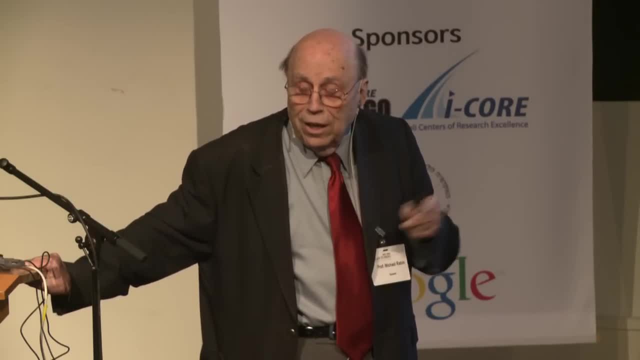 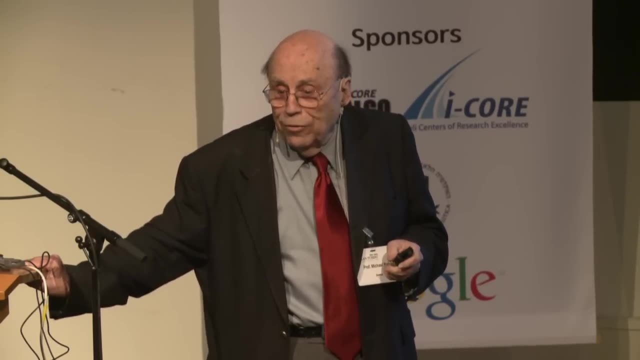 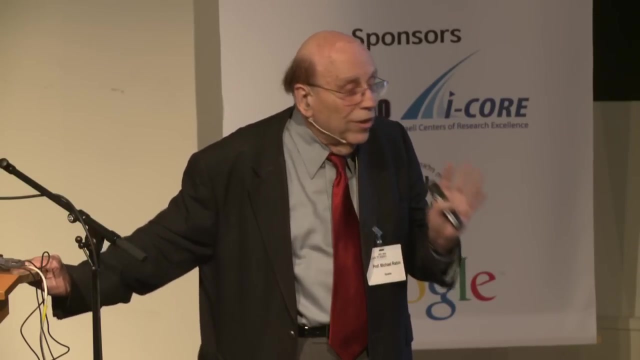 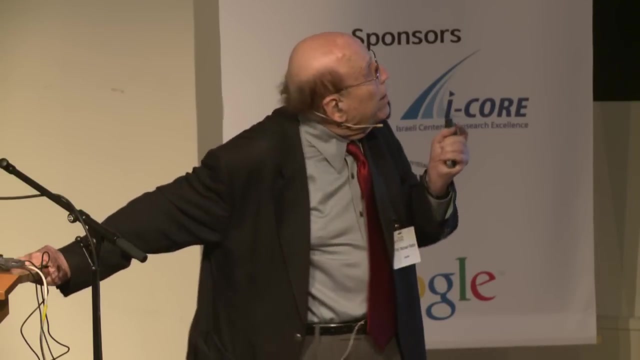 if I have a question. I'm sitting in Hawaii and I I have a question about the lecture, the Stanford lecture. there is a methodology of being able to answer these questions in a very satisfactory way. I'm not going into the details, so this is going to make this remote university education a real.